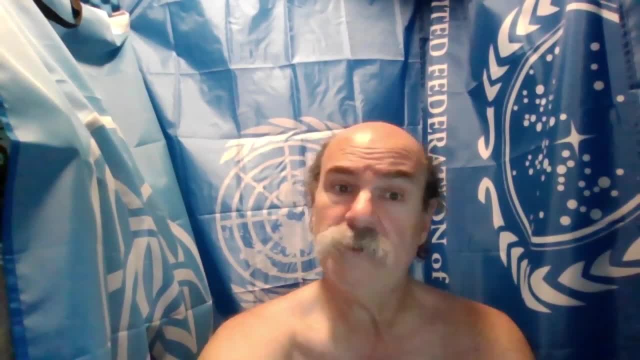 such as John von Neumann and Oskar Morgenstern in the early 20th century. Their seminal book Theory of Games and Economic Behavior laid the foundation for this field of study. There's a link to the book at the Internet Archive in the description. 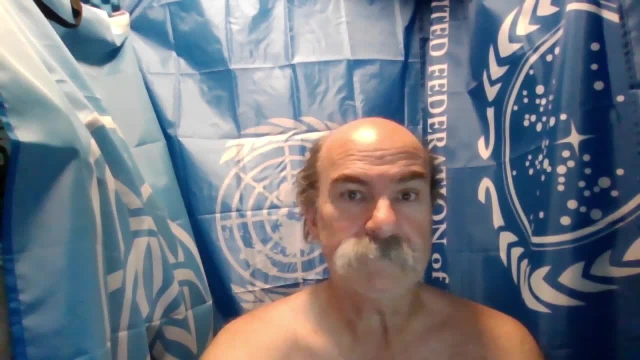 if you want to read it, Support the Internet Archive. It's a valuable resource. Originally, game theory focused on understanding strategic interactions in economics, but it quickly expanded its reach to various disciplines including political science, biology, psychology and computer science. Today it stands as a multidisciplinary field. 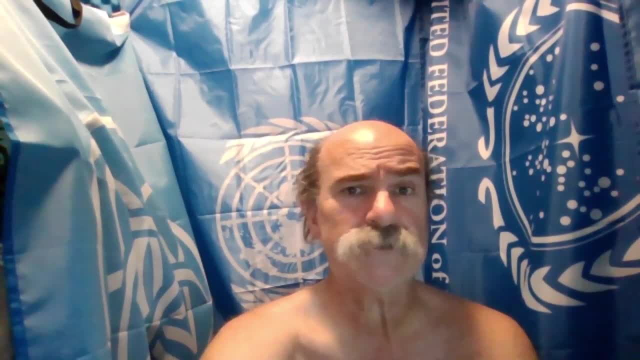 that offers valuable insights into the field of game theory. Game theory revolves around several key elements that help us analyze strategic interactions. They are players, strategies, payoffs, information and game forms. Game theory provides valuable insights across various fields like economics and finance. 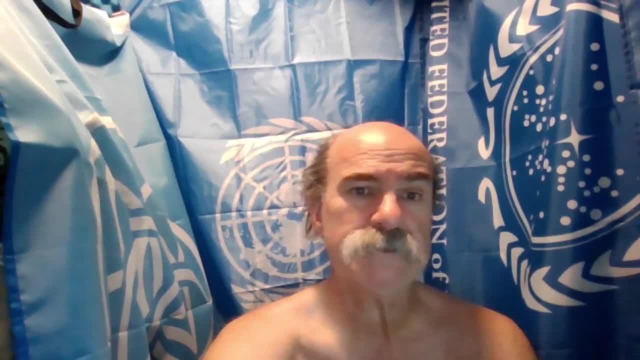 business strategy, political science and international relations, and biology and evolution. While game theory offers valuable insights into the field of game theory, it also provides powerful insights. It's important to recognize its limitations and criticisms. Some of the concerns include the simplified assumptions about human behavior. 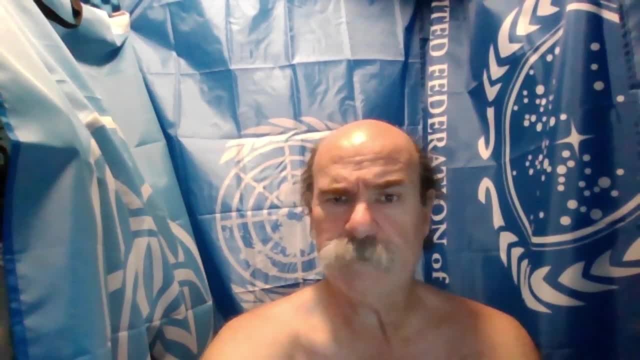 challenges in predicting real-world actions accurately and the potential to neglect broader ethical considerations. By acknowledging these limitations, we can approach game theory with a critical lens and use it alongside other analytical tools and empirical evidence, Now that we've set the stage for our exploration. 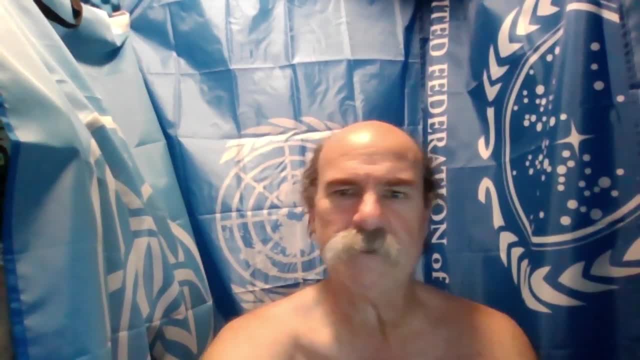 we can dive deeper into each concept and its applications. Join us as we unravel the intricacies of strategic decision-making and discover how game theory can inform our understanding of the world around us. But first let's take a step back and explore the history and 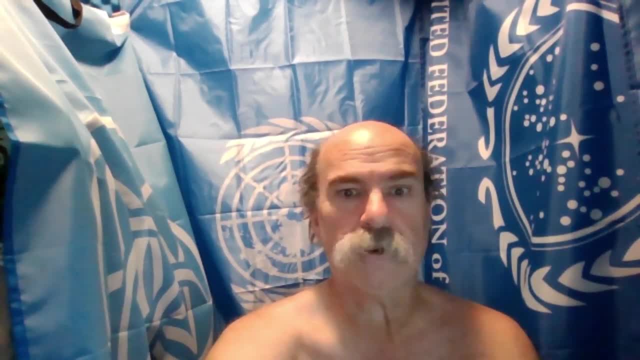 origin of game theory to gain a solid foundation for our journey. Game theory has a rich history that dates back to the early twentieth century, with its roots in economics, mathematics and political science. The development of game theory can be attributed to the groundbreaking contributions of several scholars. One of the key figures in the history of game theory is mathematician Emile Borel who, in the early 1920s, introduced the concepts of games of strategy and made significant contributions to the field. However, it was the work of mathematicians John von Neumann and Oskar Morgenstern the first we 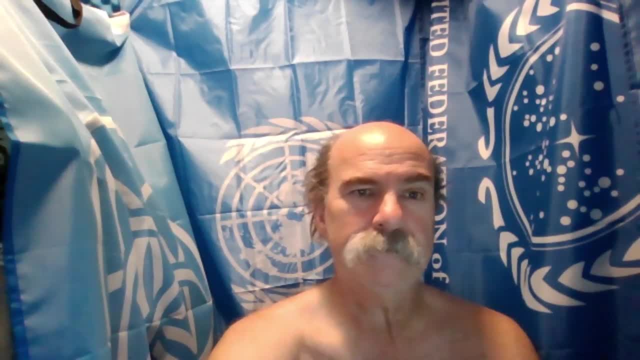 saw in game theory that made the most sense of game and political science, Game theory that truly revolutionized game theory. In 1944, von Neumann and Morgenstern published their influential book Theory of Games and Economic Behavior. which laid the foundation for modern game theory. This seminal work not only presented the mathematical models for strategic decision-making, but also introduced concepts like utility theory and the mini-max theorem. The book's impact extended beyond the fields of economics, influencing other disciplines such as political science. 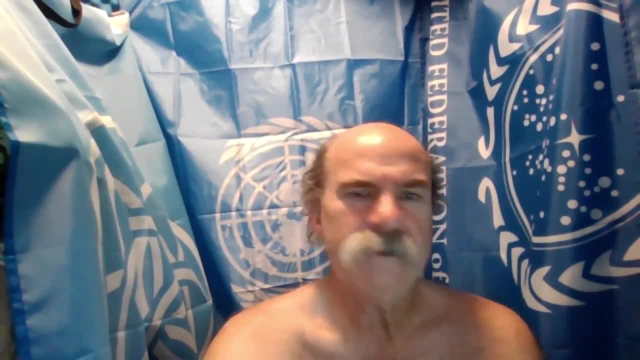 biology and computer science. Since then, game theory has continued to evolve, with contributions from numerous scholars and researchers. Game theory has proven to be an invaluable tool in understanding strategic interactions, whether it's analyzing competitive markets, predicting behavior in political negotiations or studying biological phenomena such as evolutionary dynamics. 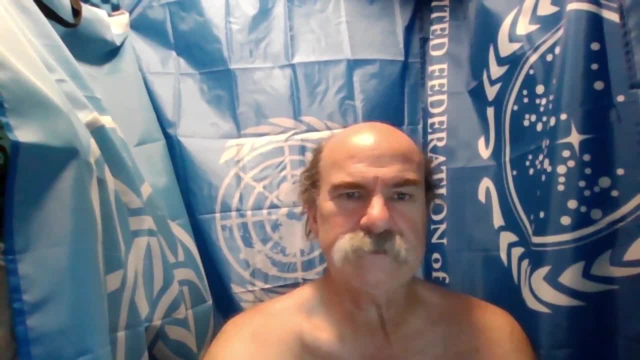 It's application and its implications have extended into various domains, demonstrating its universal relevance. By studying the origins of game theory, we can gain deeper appreciation for the intellectual journey and collaborative efforts that have shaped this fascinating discipline. It serves as a reminder that game theory is not merely a mathematical abstraction. 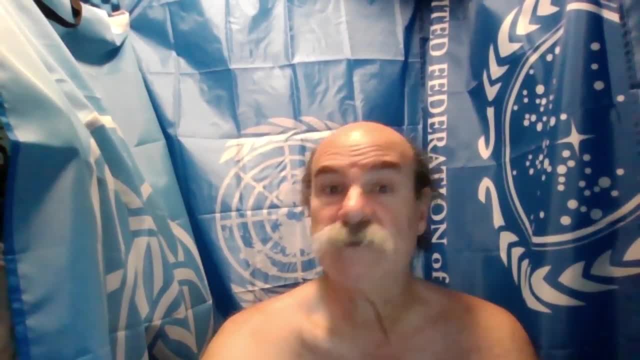 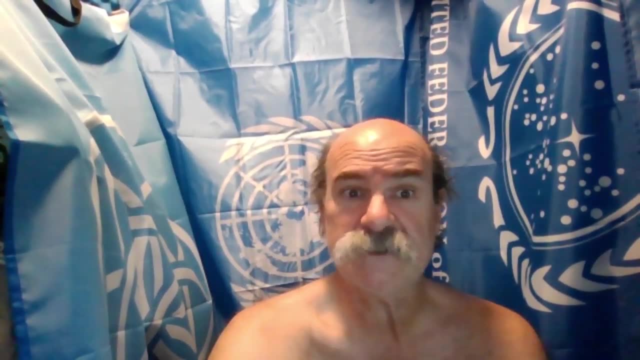 but a framework that helps us navigate the complexities of decision-making in diverse fields. Understanding the historical context of game theory also allows us to appreciate the immense progress made and the ongoing advancements that continue to push the boundaries of our knowledge As we explore the concepts and applications of game theory. 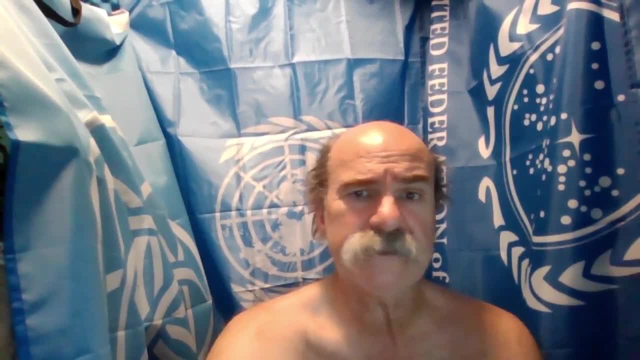 we build upon the foundation laid by the visionaries who paved the way for this captivating field of study. To fully comprehend game theory, it's essential to explore the fundamental concepts and components that form the building blocks of this field. These concepts provide a framework for analyzing strategic decision-making. 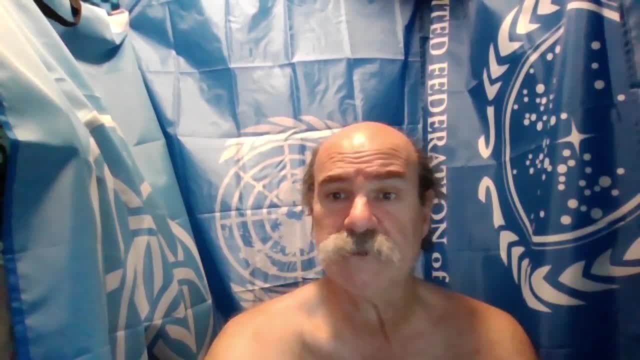 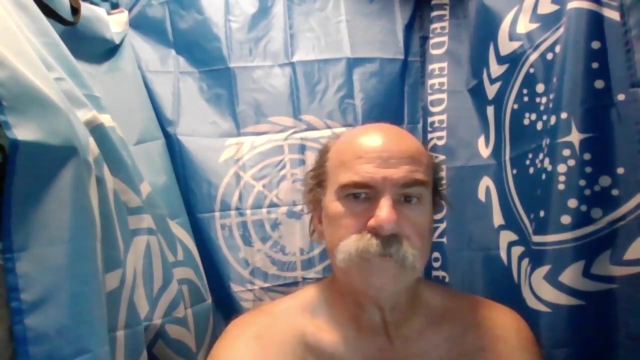 and understanding the dynamics of interactions between rational decision-makers. Players are the participants or decision-makers involved in a game. They can be individuals, groups, organizations or even nations, depending on the context of the game. Each player is characterized by their own set of preferences. 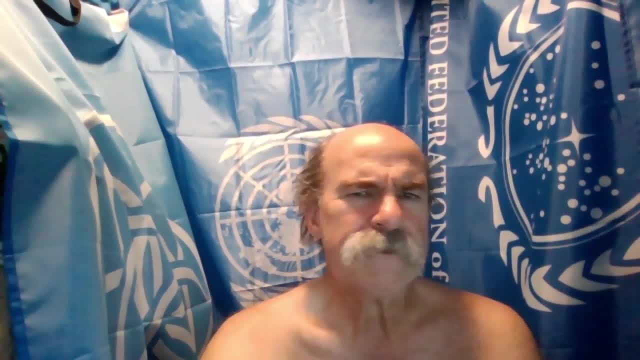 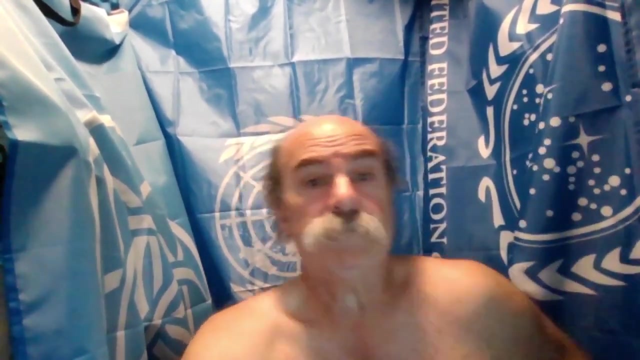 objectives and strategies. Game theory assumes that players are rational decision-makers who act in their own self-interest, aiming to maximize their own payoffs. This assumption of rationality allows for the analysis of strategic behavior and the prediction of player actions. Players in the game can also have different characteristics. 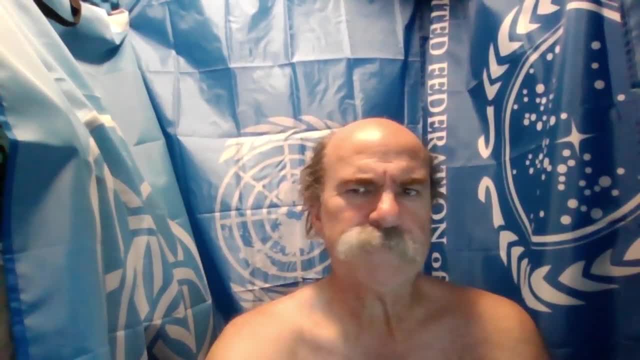 abilities, resources and preferences. These differences can lead to various strategies and outcomes. Heterogeneity among players is a key factor in game theory. Heterogeneity among players adds complexity and richness to the analysis of strategic interactions. Games can involve any number of players. 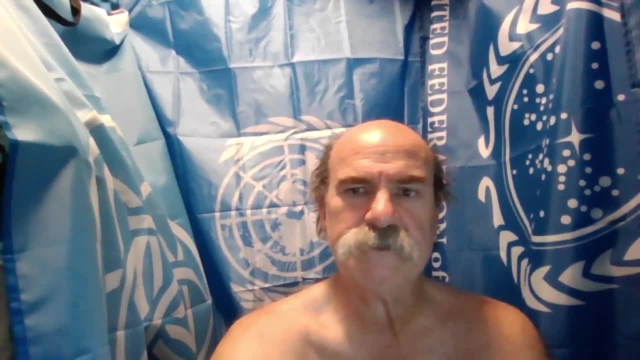 from a two-player game to situations with numerous participants. The number of players can significantly impact the dynamics and strategic considerations within a game. For example, in a two-player game, the actions of one player directly affect the other, whereas in games with many players, players may form alliances. 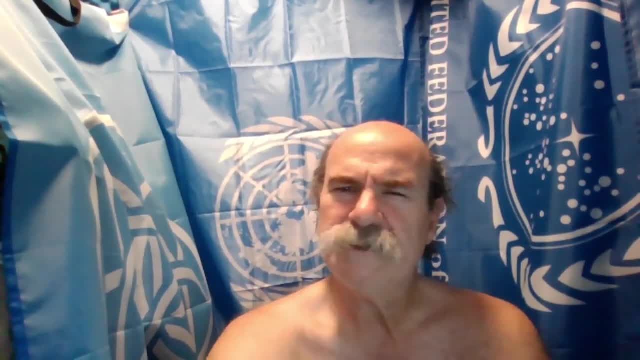 or compete with specific subsets of others. The decisions of players in the game are interdependent, meaning that the outcome for each player depends not only on their own actions, but also on the actions of other players. This interdependence leads to strategic thinking. 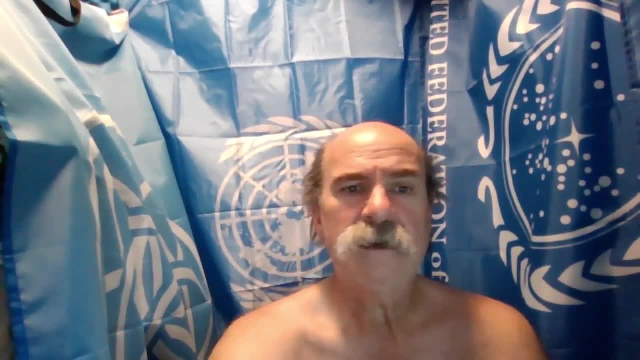 as players consider the potential actions and responses of others when making their decisions. Games can involve sequential moves, where players take turns making decisions, or simultaneously, where players act simultaneously without knowing the actions of others. The sequence of moves can influence the strategies and outcome of the game. 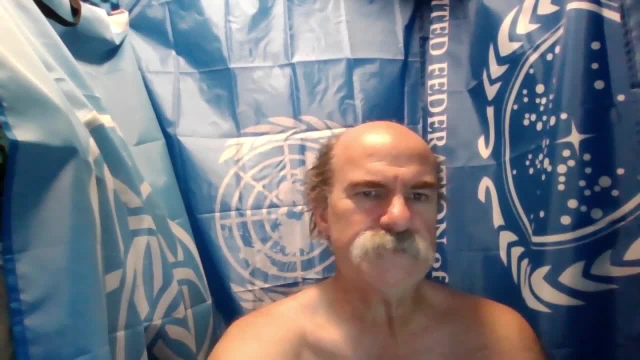 Understanding the players in the game allows us to analyze their objectives, strategies and decision-making processes. By considering the rationality, heterogeneity, interdependence and the number of players involved, we can explore the complexities of strategic interactions and predict how players might act. 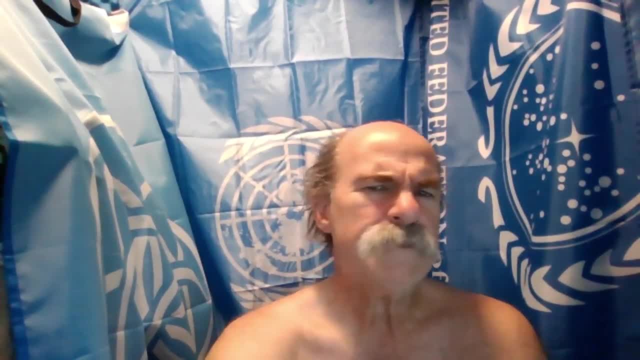 We can also study how players might behave in different situations. Game theory provides a powerful framework to study and understand behavior of players in a wide range of contexts, from competitive markets to political negotiations, to evolutionary dynamics and social interactions. By unraveling the motivations and strategies of players, 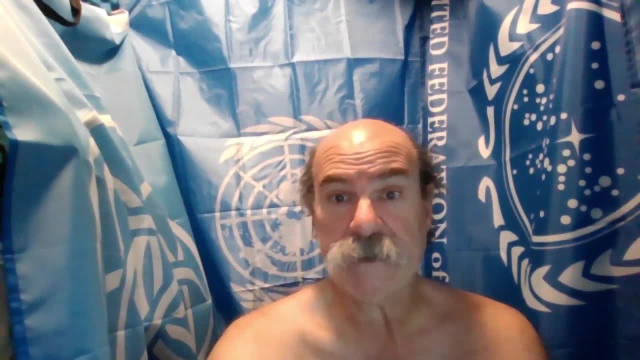 we gain valuable insights into strategic decision-making and its implications in various domains. Strategies represent the role of players in the game and they represent the choices available to each player in the game. They encompass the actions, decisions or moves that players can make to pursue their objectives. 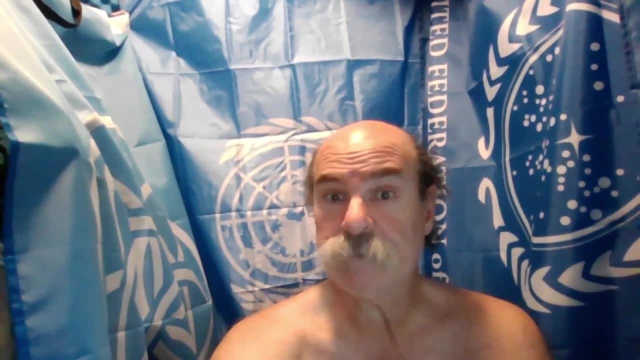 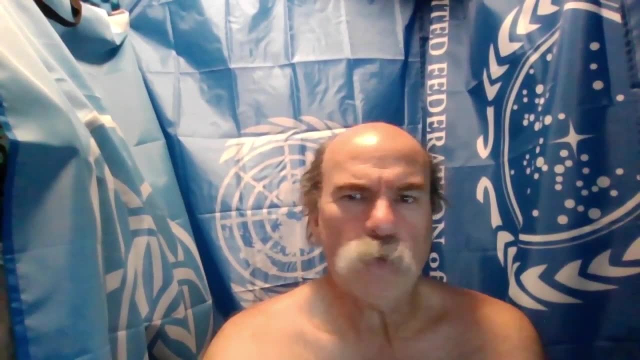 Understanding strategies is crucial for analyzing the decision-making process of players and predicting their behavior in the game. A pure strategy is a specific, well-defined choice or action that a player can take in a game. It is a simple, unambiguous decision made by a player. 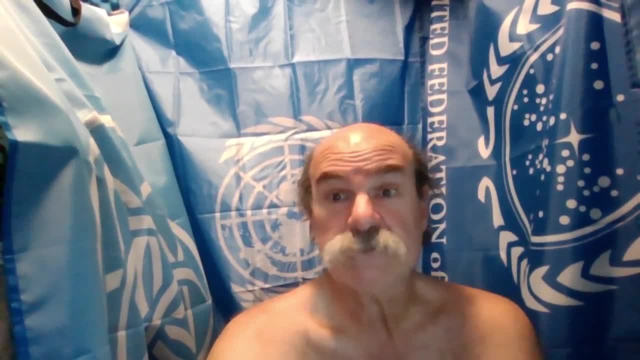 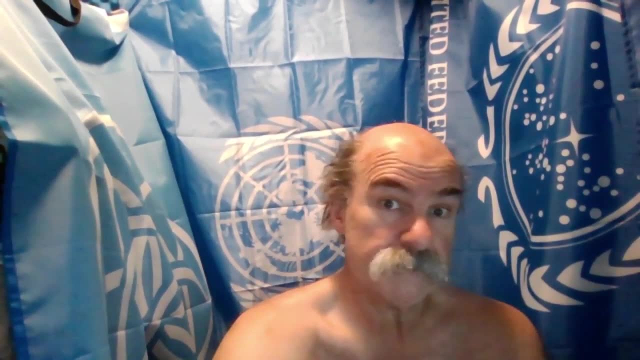 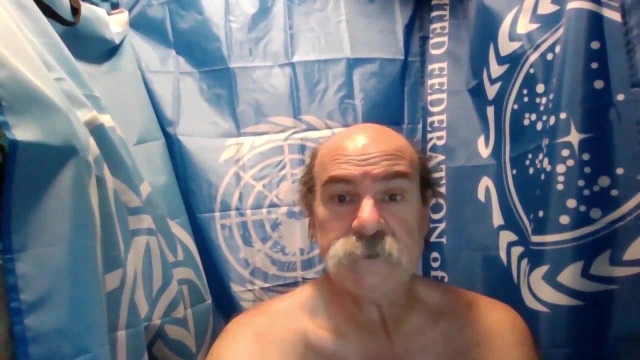 For example, in a game of rock paper, scissors- lizard- Spock, the pure strategies for each player are to choose rock paper, scissors, lizard or Spock. In some games, players may employ mixed strategies, which involves probabilistic or randomized choices. 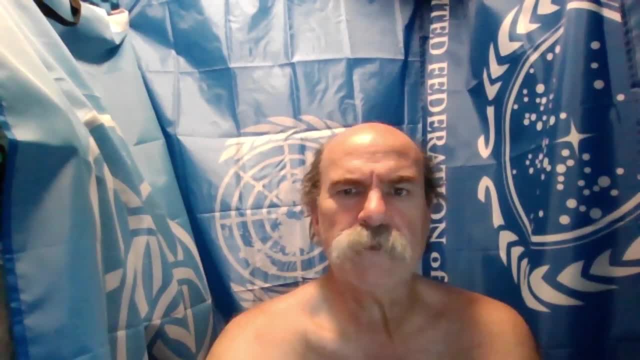 A mixed strategy represents a probability distribution over the pure strategies available to the player. Players may randomize their decisions to introduce uncertainty and unpredictability, making it more challenging for opponents to anticipate their actions. A dominant strategy is a strategy that provides a player with the highest payoff. 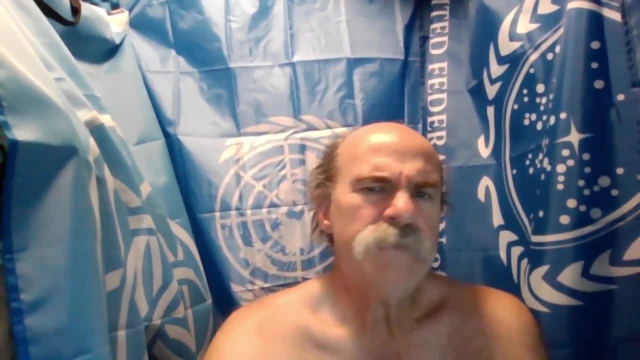 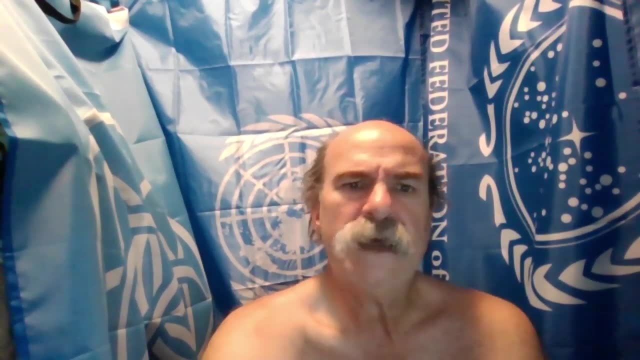 regardless of the actions taken by other players. If a player has a dominant strategy, it's the best choice, regardless of the strategies chosen by opponents. Dominant strategies simplify the analysis of games, as players can confidently select the strategy that maximizes their payoff. 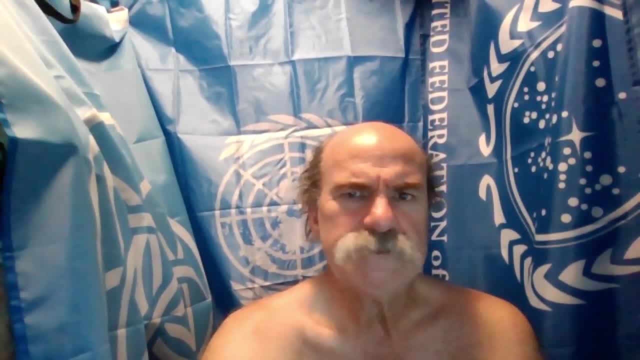 A best response strategy is one that maximizes a player's payoff. given the strategies chosen by other players, It represents the optimal choice for a player based on their beliefs about the actions of others. Players aim to select the best response strategy to optimize their outcome within a game. In game theory, strategies are influenced by the actions and choices of other players. Players consider the potential strategies and responses of others when selecting their own strategies. The interplay of different strategies and their interactions form the dynamics of strategic decision-making in a game. 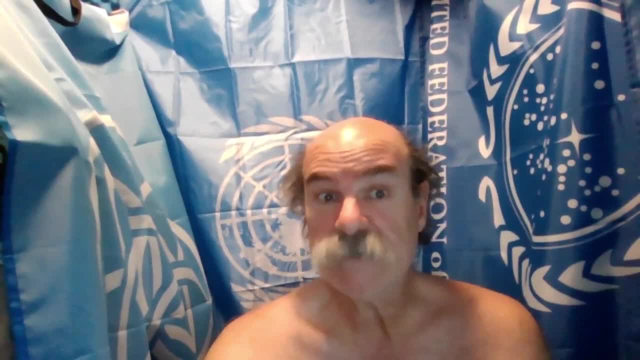 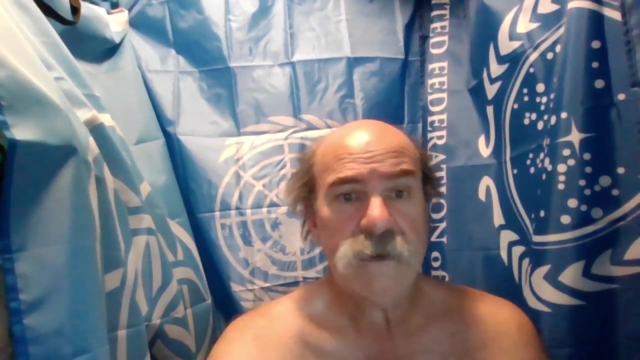 Game theory explores equilibrium concepts such as Nash equilibrium, where no player has an incentive to unilaterally deviate from their chosen strategy. Equilibrium strategies represent stable states in a game where players find a balance between their own objectives and the anticipated outcome. 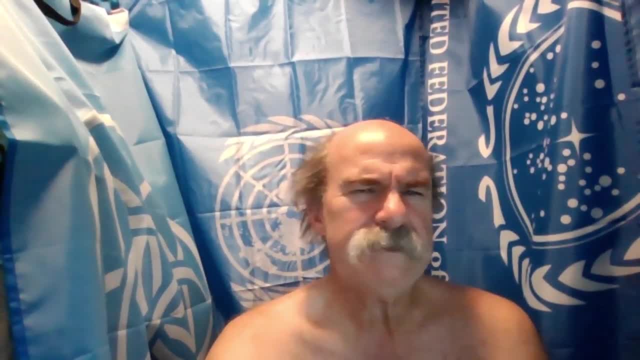 Game theory also explores the potential outcome of a game and the strategies that lead to favorable results. By analyzing the available strategies and their implications, game theory provides insights into the decision-making process of players, the potential outcome of a game and the strategies that lead to favorable results. 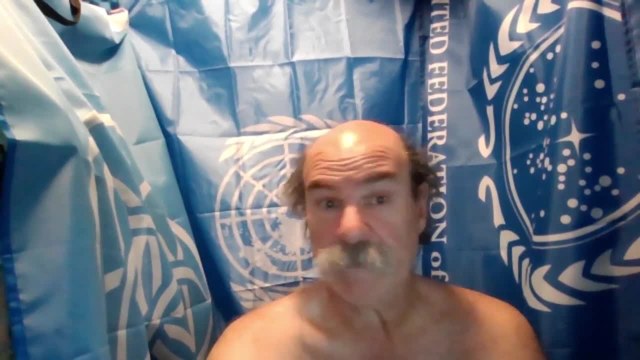 Understanding a range of strategies, from pure strategies to mixed strategies, allows for a comprehensive examination of strategic interactions and the complexities of decision-making in different contexts. Game theory's analysis of strategies provides a powerful framework to study competitive behavior, negotiate outcomes and make informed decisions in a wide range of fields. 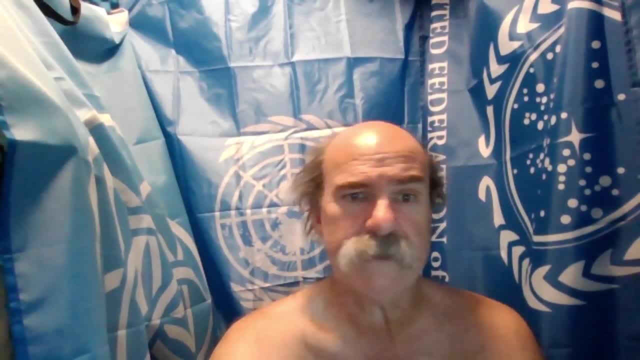 including economics, politics, biology and social sciences. By unraveling the strategic choices available to players, we gain valuable insights into their decision-making processes and the dynamics of strategic interactions. Payoffs are the outcome of strategic interactions. Payoffs are the outcome of strategic interactions. 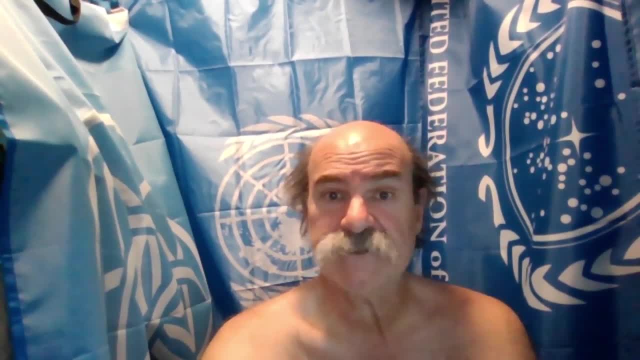 They represent systemic outcome or rewards associated with specific combinations of choices made by the players in a game. They represent the players objectives and provide a basis for evaluating the success or desirability of different outcomes. Understanding payoffs is crucial for analyzing strategic decision-making. 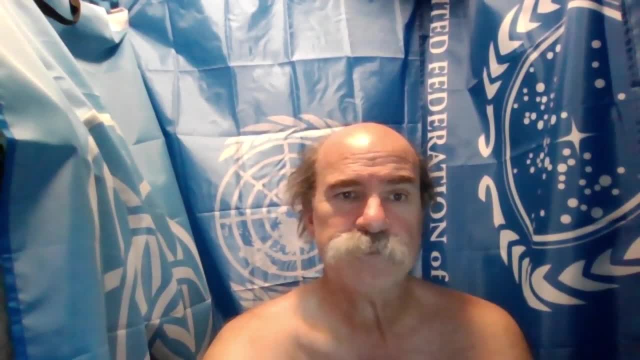 and assessing the consequences of different strategies. Payoffs are often measured in terms of utility, which represents the subjective value or satisfaction of player. decision-making derives from a particular outcome. Utility can be influenced by various factors, such as financial gains or losses, emotional well-being, social status or other individual preferences. 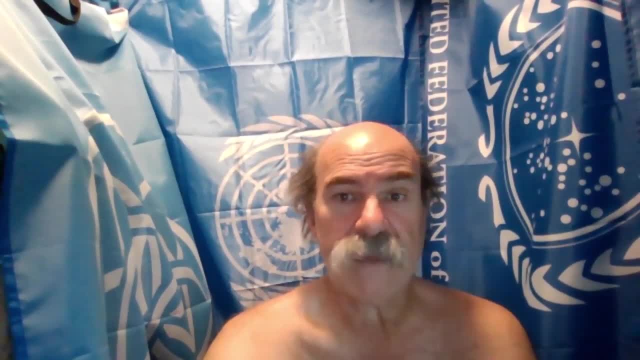 Payoffs can be positive or negative, depending on the nature of the game and the objectives of the players. Positive payoffs indicate favorable outcomes, such as monetary gains, rewards or benefits. Negative payoffs represent undesirable outcomes, such as losses, penalties or costs. 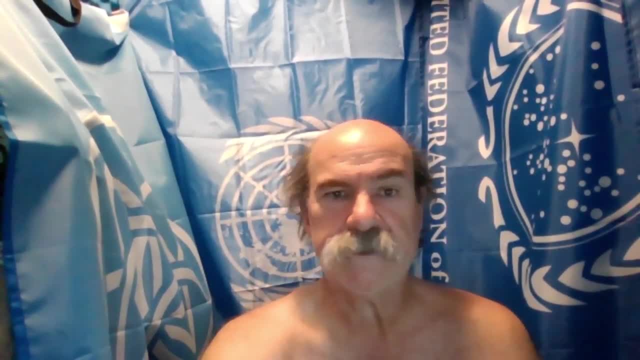 In multiplayer games, payoffs are typically represented in a payoff matrix, which shows the payoffs for each player based on the combination of strategies chosen by all players. Each cell of the matrix corresponds to a specific combination of choices and represents respective payoffs for the players involved. 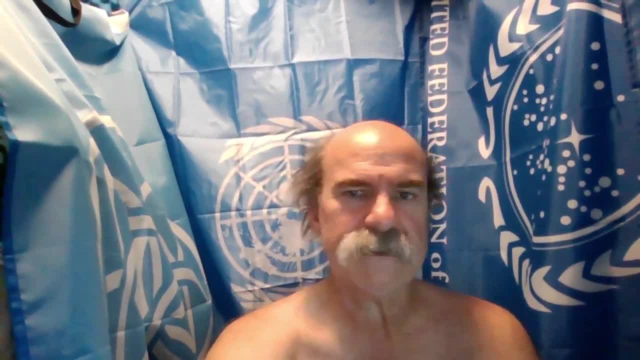 Payoffs can be informative. Payoffs can be interpreted differently depending on the context of the game. In competitive games, players can maximize their own payoffs relative to the payoffs of other players. In cooperative games, players can strive for fairness or the maximization of. 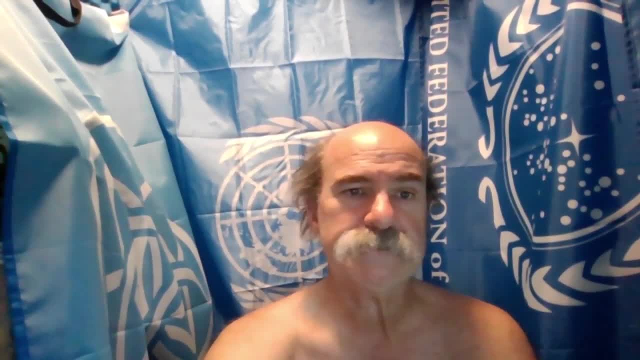 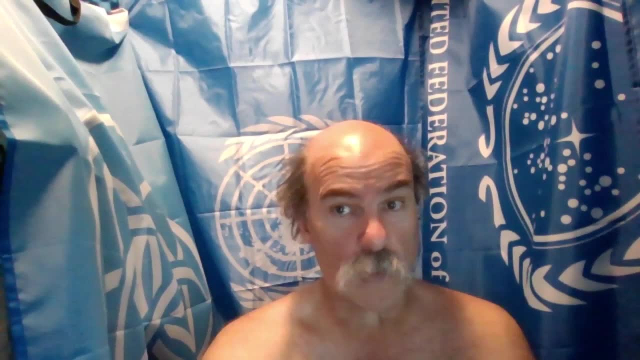 collective payoffs through collaboration and coordination. A Pareto-efficient outcome is one where no player can be made better off without making another player worse off. It represents an allocation of payoffs that is considered optimal where no alternative application would improve the situation for at least one player without 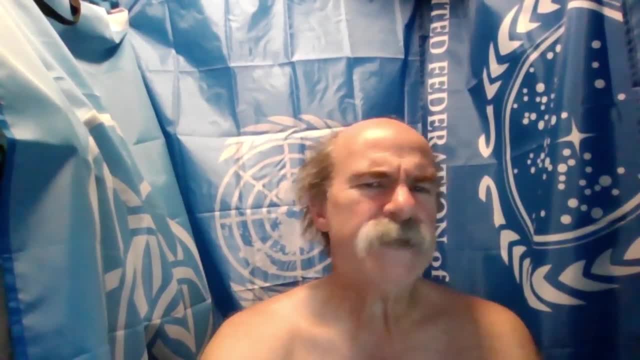 reducing the outcome for another. Understanding payoffs allows us to evaluate the desirability of different outcomes, predict player behavior and analyze the incentives that drive strategic decision-making. By examining the utility, positive and negative implications, payoff matrices and interpretations of payoffs, game theory provides a framework for assessing the consequences of a decision-making. 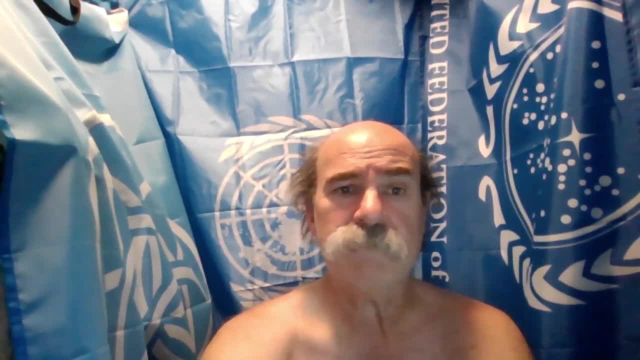 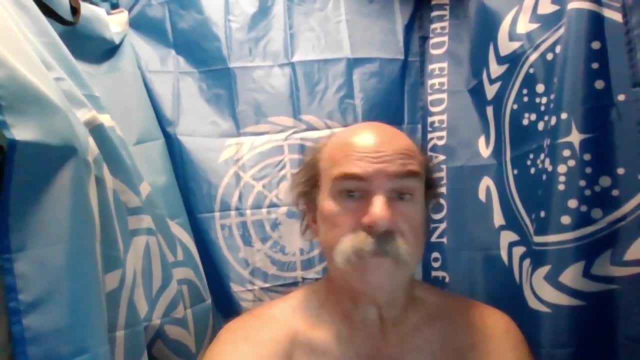 and looks like moves, expectations and needs for performance. The analysis of the match-up in game theory has practical applications in fields such as economics, business, social sciences and beyond. By unraveling the incentives and rewards associated with different choices, we gain insight into how players make decisions. the 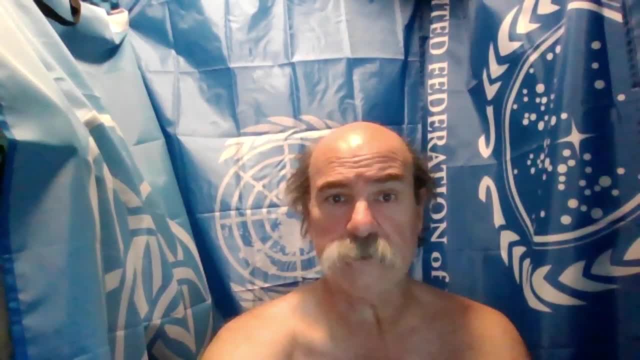 tradeoffs they face and the potential outcomes that emerge from their interactions. Ultimately, the answers are quite simple: 1. Comprehensive- A cetera pulls a player out of a helped-". 2. Understands target effects. 6. Punish the versus misper reviewed. 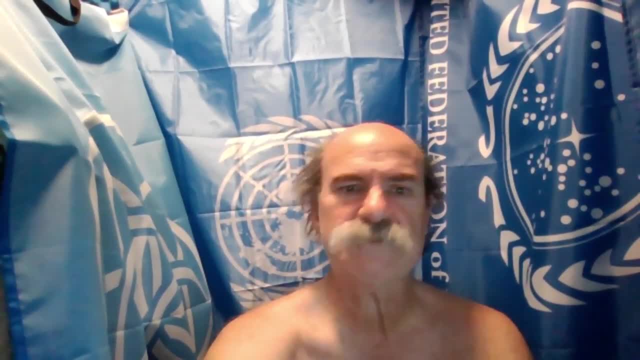 Understanding payoffs helps us navigate the complexities of strategic decision-making, optimize outcomes and explore the dynamics of interactions between rational players in a wide range of scenarios. Information plays a crucial role in game theory. It refers to what each player knows about the game, the strategies of other players, 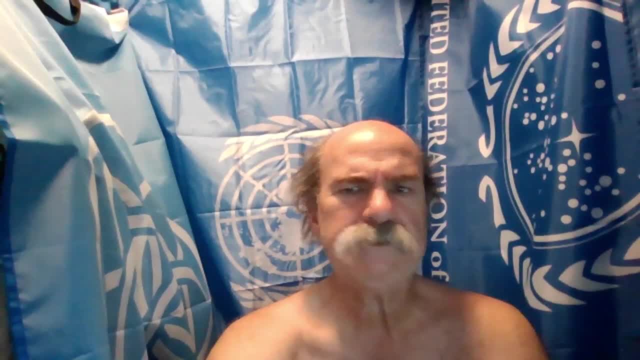 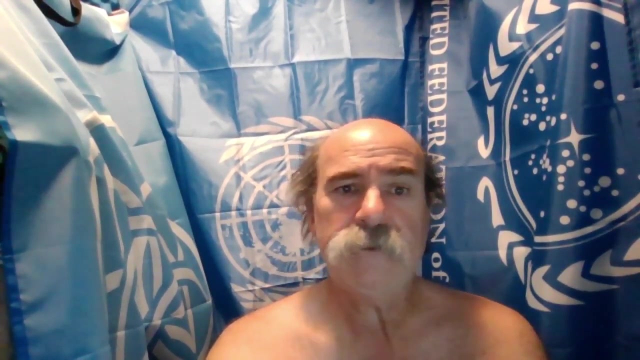 and the potential payoffs. The level of information can vary in different games, ranging from complete information to incomplete or imperfect information. In games with complete information, each player has perfect knowledge about the structure of the game, the available strategies and the payoffs associated with different outcomes. 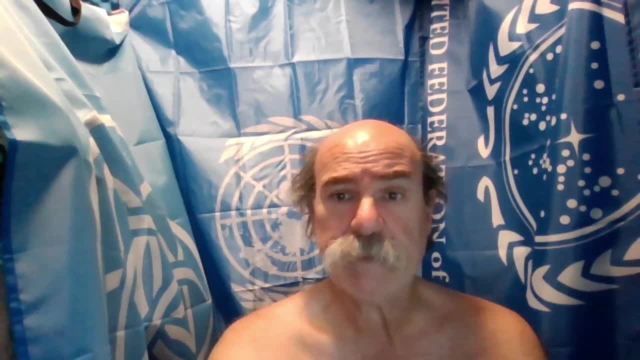 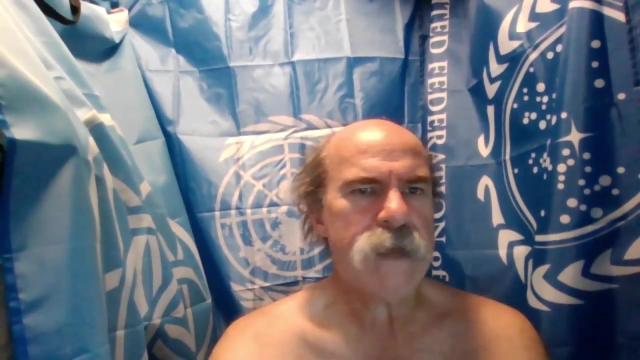 Players know the actions taken by others and make decisions based on this complete knowledge. In many real-world situations, players have limited or imperfect information about the game and the strategies chosen and the strategies taken by others. In games with incomplete information, players may not know certain aspects of the game. 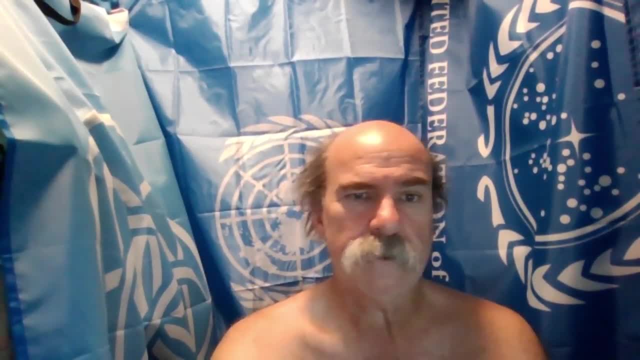 such as the private information held by other players, the preferences of other players and the exact payoffs associated with different outcomes. Private information refers to information that is known only to specific players. This information can significantly impact the strategies and decisions of players. 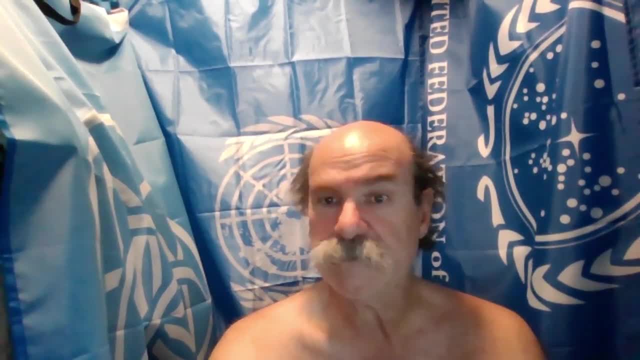 Players with private information may have an advantage, as they can tailor their strategies based on their unique knowledge. In sequential games, players make decisions in a specific order and the information available to each player may change as the game progresses. Information sets represent the knowledge that a player has at a particular point in the game. 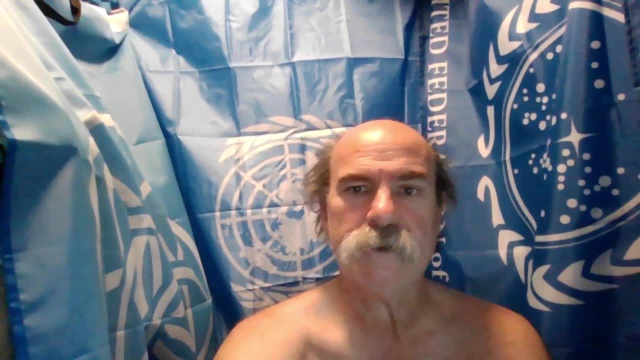 including their own actions and the actions of others. up to that point, Players make decisions based on their information sets. Games with perfect information are those in which players have complete knowledge of the moves made by all players and the consequences of those moves. On the other hand, games with imperfect information involve uncertainty. 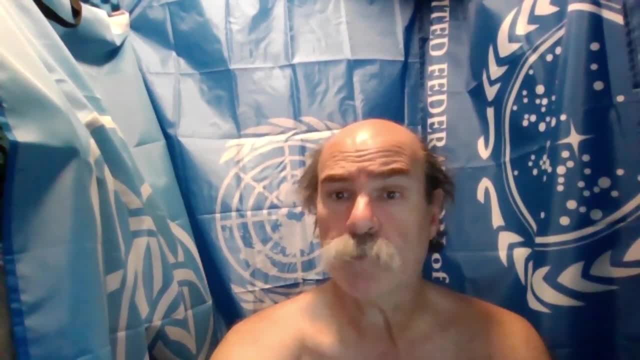 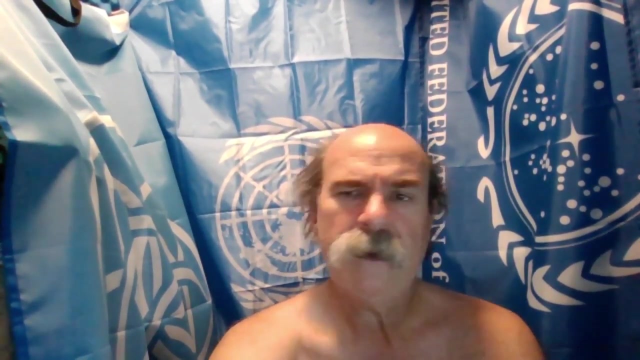 as players lack full knowledge of the actions or private information of others. Information asymmetry occurs when some players have more information than others in the game. This disparity can lead to strategic advantages for players with greater knowledge, as they can use it to make better informed decisions. 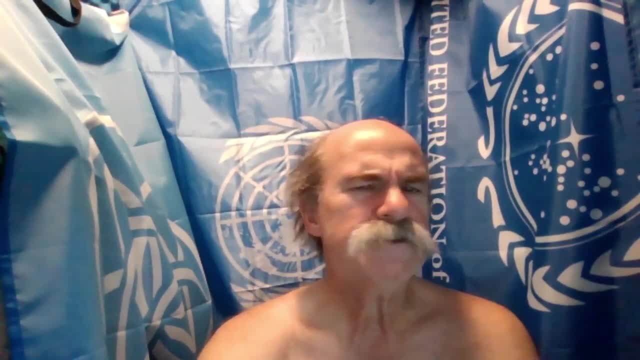 and gain an edge over opponents. Understanding the role of information in game theory helps us: analyze strategic decision-making in realistic scenarios. The level of information influences the strategies players choose, the outcomes they anticipate and the dynamics of the game, Analyzing how players acquire, process and use information. 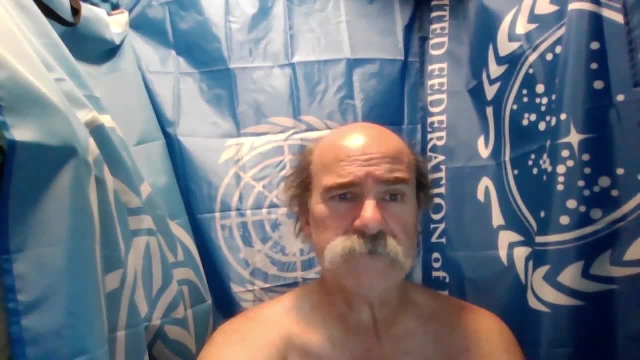 provides valuable insights into the strategic considerations and interactions that shape the decision-making process. Game theory explores various information structures and their impact on strategic behavior. By studying complete and incomplete information, private information, information sets and the asymmetry of information, we gain a deeper understanding of how information influences outcomes strategies. 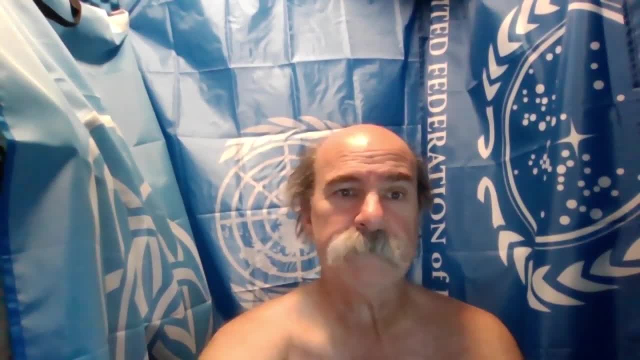 and the complexities of strategic interactions. In practice, game theory allows us to navigate situations where information is limited or uncertain, such as negotiations, auctions or competitive markets. By unraveling the role of information, game theory equips us with tools to make informed decisions, anticipate the actions of others. 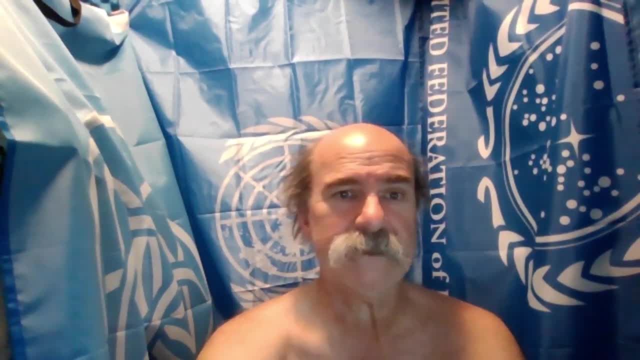 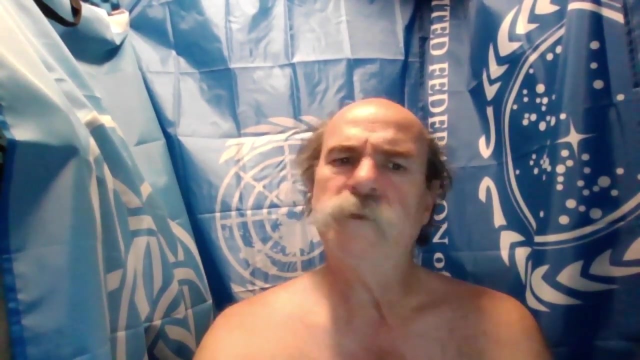 and strategize effectively in diverse contexts. Game forms define the rules and constraints of a particular game. They specify the set of players, their strategies, the order of moves and the information available to each player. Different game forms can result in distinct outcomes and strategic considerations. 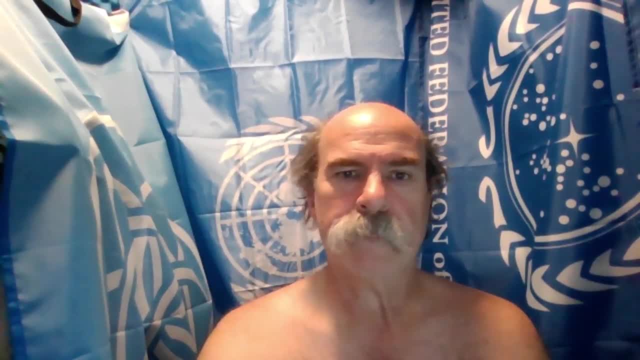 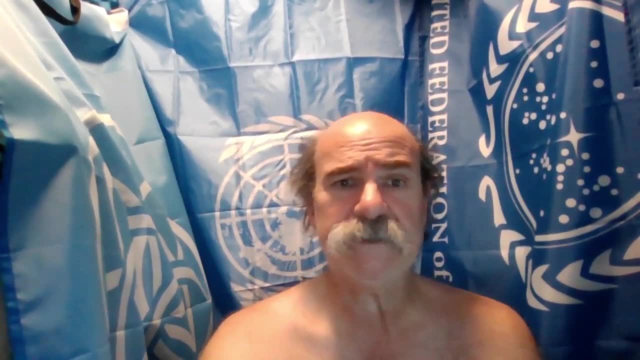 Let's explore some of the common types of game forms. Normal form games, also known as strategic form games, represent games where players make simultaneous decisions without knowing the choices of others. The game is typically represented in a matrix form, known as a payoff matrix. 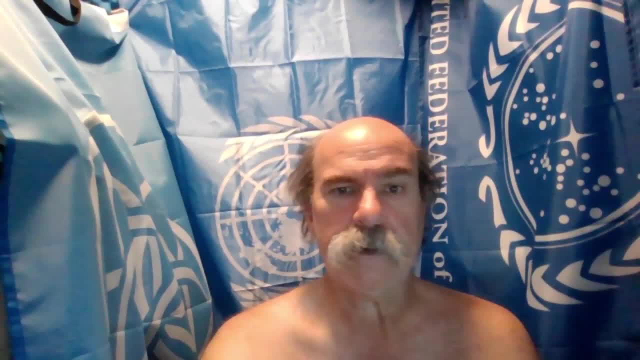 where each cell represents the payoffs for each player based on their strategies. Extensive form games capture sequential decision making, where players make choices in a specific order, possibly with the ability to observe previous actions. These games are represented as a game tree. 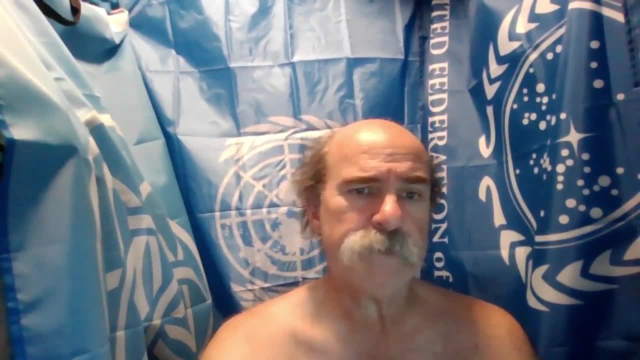 where nodes represent decision points, branches represent possible choices and terminal nodes represent the outcomes and associated payoffs. Cooperative games involve players forming coalitions and working together to achieve joint outcomes. In these games, players negotiate, make arrangements and distribute payoffs among the members of the coalition. Cooperative game theory focuses on analyzing the fairness and efficiency of different allocation mechanisms. In symmetric games, all players have identical sets of strategies and payoffs. These games involve identical players who face the same strategic choices and outcomes. In asymmetric games, players have distinct sets of strategies and payoffs. 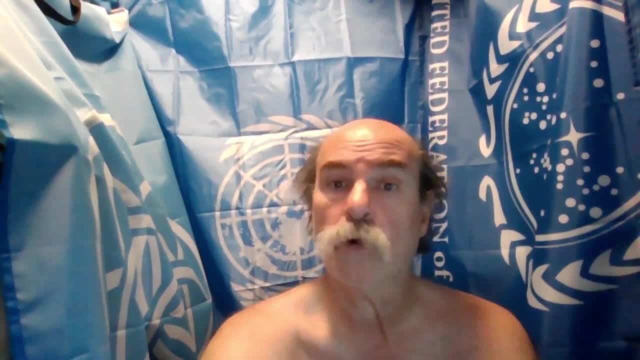 reflecting their individual characteristics, roles or positions. Static games involve a single round of decision making, where players make simultaneous choices without the ability to observe or react to others' actions. Dynamic games, on the other hand, incorporate multiple rounds of decision making. 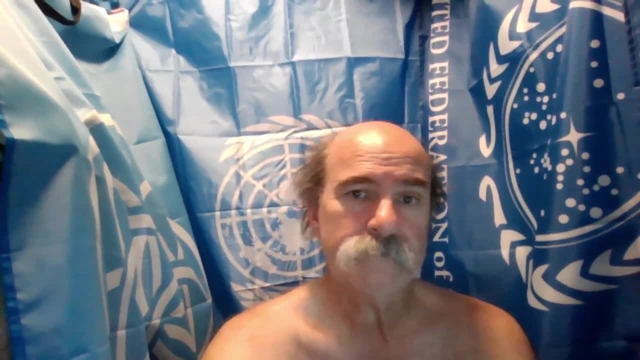 allowing players to observe and respond to the actions of others. Repeated games involve the repetition of a particular game over multiple rounds or an indefinite number of times. The outcomes and payoffs of previous rounds can influence the strategies and decisions made in subsequent rounds. 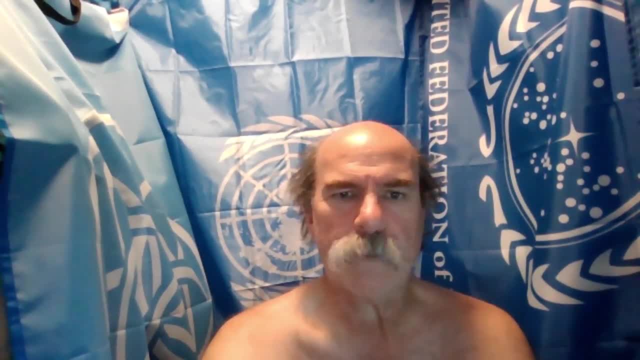 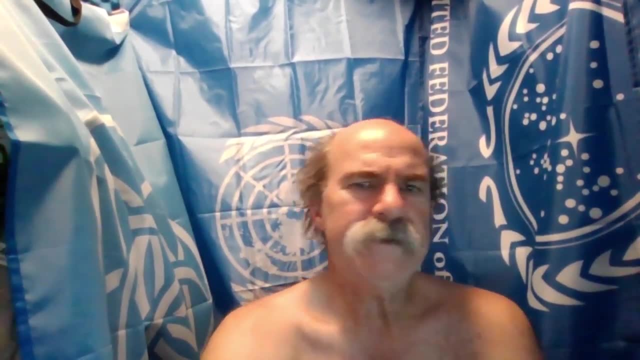 Repeated games provide insights into the dynamics of cooperation, reputation and the possibility of establishing long-term strategies. Understanding different game forms helps us analyze the structure, dynamics and strategic considerations of a game By examining normal game forms, extensive game forms. 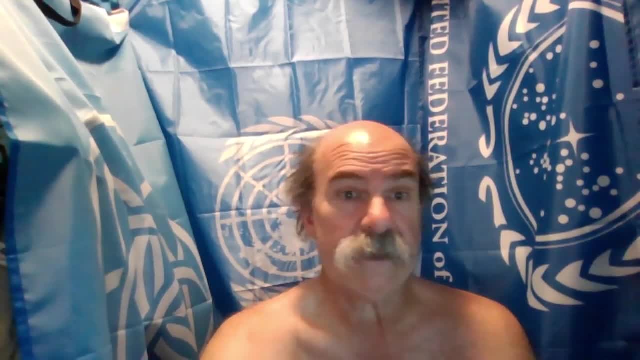 cooperative games, symmetric and asymmetric games, static and dynamic games and repeated games, we can gain insights into the complexity and diversity of strategic interactions. Game theory provides a framework to study and analyze various game forms, allowing us to predict outcomes, determine optimal strategies. 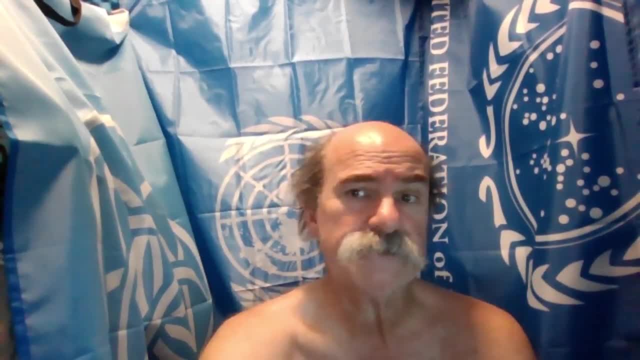 and explore the implications of different decision-making structures. By unraveling the rules, constraints and information available in different game forms, we can better understand the strategic interactions and decision-making processes in a wide range of scenarios. Equilibrium concepts in game theory allow us to analyze stable outcomes. 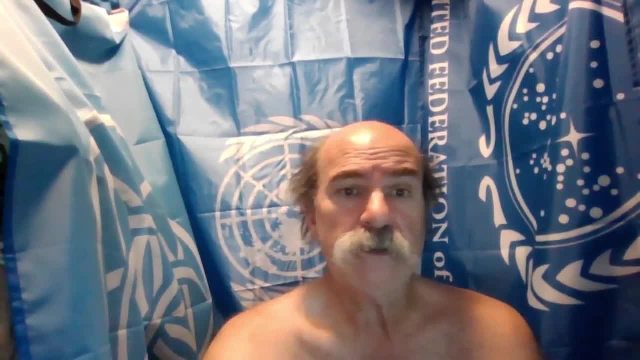 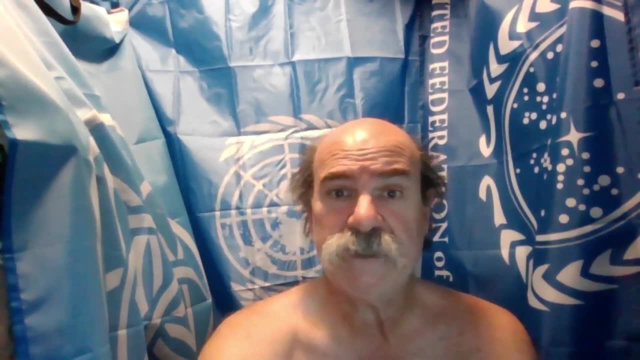 where no player has an incentive to unilaterally deviate from their chosen strategy. These concepts provide valuable insights into the strategic decision-making of players and the potential outcomes of the game. Here are some common equilibrium concepts: The Nash equilibrium is one of the most widely studied. 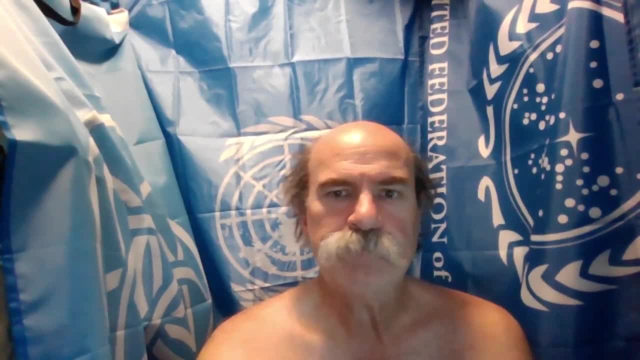 equilibrium concepts in game theory. It represents a state in a game where no player can improve their payoff by changing their strategy, assuming that all other players remain unchanged. In a Nash equilibrium, each player's strategy is the best response to the strategy chosen by others. 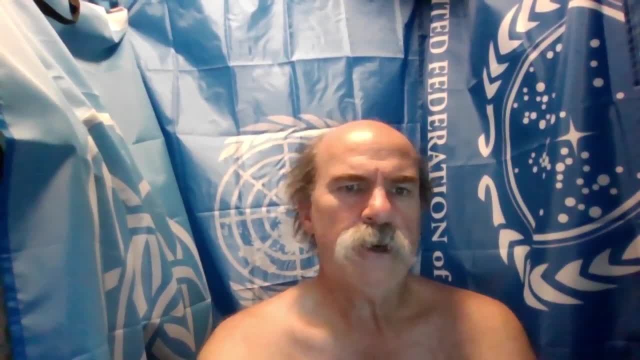 A dominant strategy equilibrium occurs when every player in the game has a dominant strategy. A dominant strategy is a strategy that provides the highest payoff for a player, regardless of the actions taken by other players. In a dominant strategy equilibrium, all players choose their dominant strategy, leading to a unique outcome. In some games, players may employ mixed strategies, which involve randomizing their choices based on probabilities. A mixed strategy equilibrium is reached when each player's mixed strategy is optimal given the strategies chosen by others. It represents a balance of randomization where no player can improve their payoff. 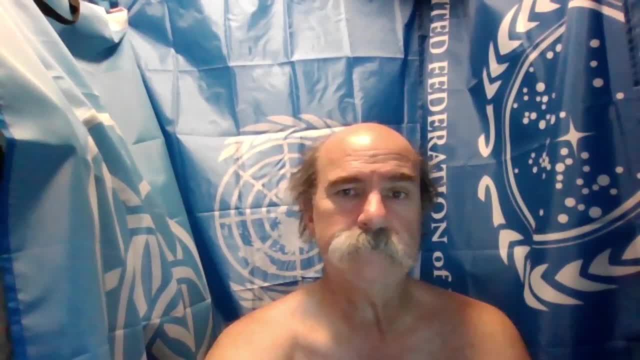 by unilaterally changing their probabilities. Subgame perfect equilibrium applies to extensive forum games and represents a strategy profile that constitutes a Nash equilibrium in every subgame of the original game. A subgame is a subset of the overall game that starts at a particular decision node. 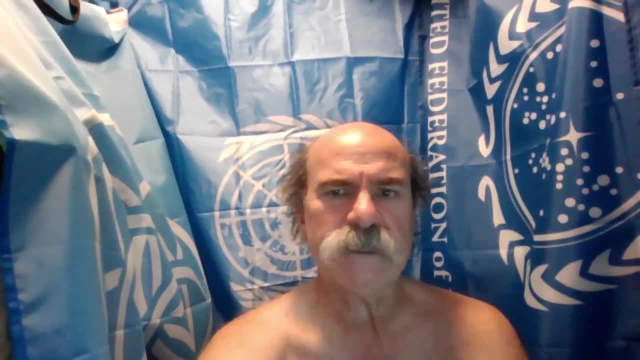 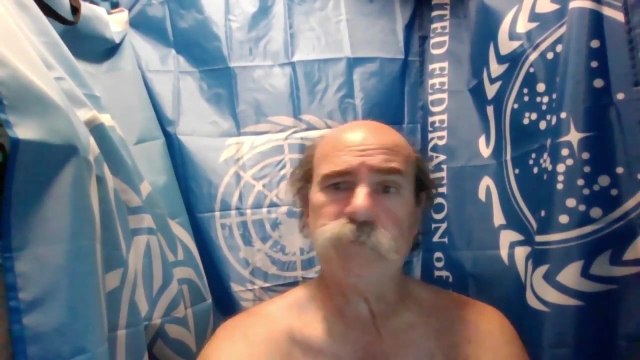 A subgame. perfect equilibrium ensures that a player's strategy is consistent throughout the game, even in subgames that occur at different points. Evolutionary game theory examines the long-term stability of strategies in populations of players. An evolutionary stable strategy, or ESS. 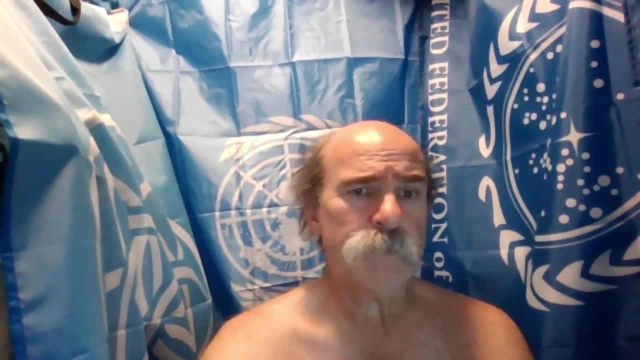 is a strategy that, if adopted by a significant proportion of the population, cannot be invaded by alternative strategies. ESS explores the dynamics of strategies, evolution and natural selection over time. Understanding equilibrium concepts allows us to predict and analyze the outcomes of strategic interactions in a game. Nash equilibrium provides insights into stable outcomes based on a player's best response, while dominant strategy equilibrium focuses on the existence of dominant strategies, Mixed strategy equilibrium considers the optimal randomization of strategies and subgame perfect equilibrium analyzes consistent strategies throughout an extensive form game. 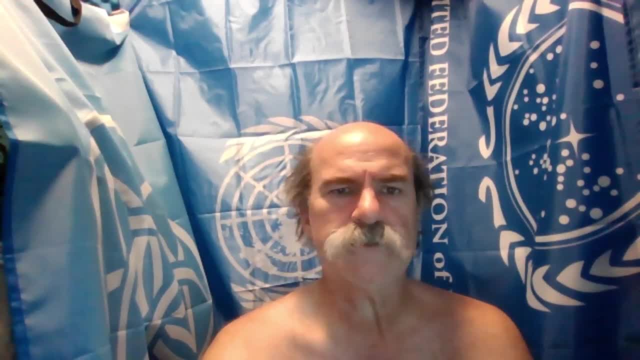 Evolutionary stable strategies explore long-term stability of strategies in evolving populations. Equilibrium concepts provide valuable tools for understanding decision-making and predicting outcomes in a wide range of scenarios, from economic markets and social interactions to political negotiations and evolutionary dynamics. By examining these equilibrium concepts, 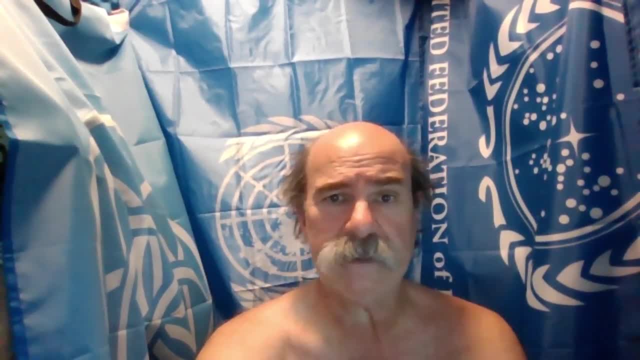 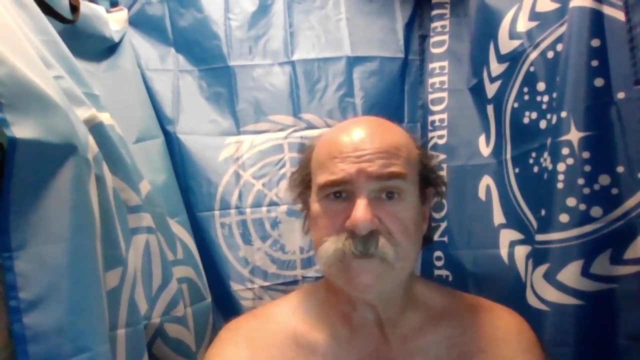 we gain insights into the rational decision-making of players and the stability of strategic interactions in various contexts. Understanding these fundamental concepts allows us to analyze strategic interactions, predict outcomes and evaluate the decision-making processes of rational players. Game theory provides a systemic framework to model complex scenarios. 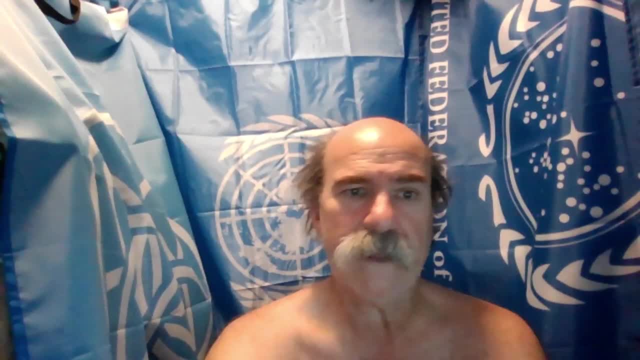 and uncover the strategies that lead to desirable outcomes. By grasping these foundational elements of game theory, we can navigate the intricate dynamics of strategic decision-making and gain valuable insights into a wide range of fields, including economics, politics, biology and beyond. 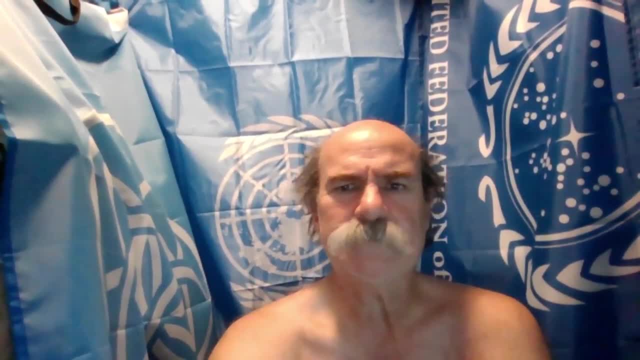 In addition to the fundamental concepts we've discussed, game theory also offers us a glimpse into classic scenarios that have captured the imagination of researchers and enthusiasts alike. These scenarios represent the strategic interactions that have been extensively studied and analyzed. Let's explore some of the intriguing classic game theory scenarios. 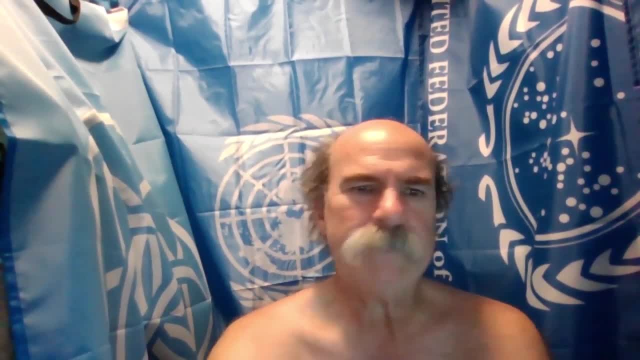 The Prisoner's Dilemma is perhaps the most well-known and extensively studied scenario in game theory. It depicts a situation where two individuals are arrested and interrogated separately, With limited communication between them. each prisoner faces a choice between cooperating with their partner. 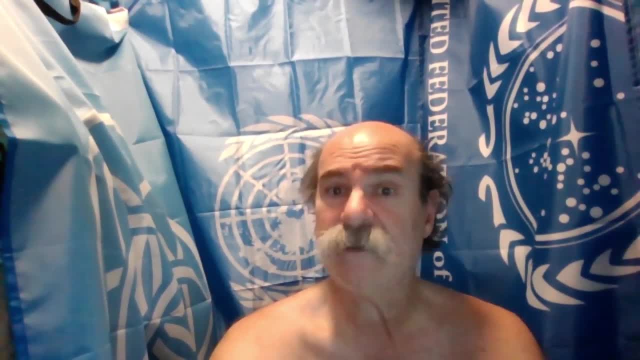 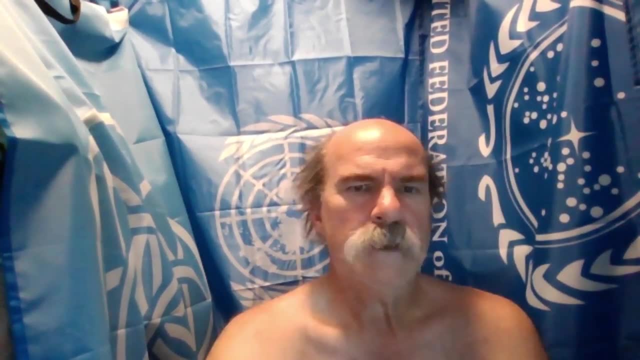 by remaining silent or betraying their partner by confessing to the crime. The outcome of the Prisoner's Dilemma can be represented as follows: If both prisoners remain silent, if they cooperate with each other, they each receive a moderate sentence. 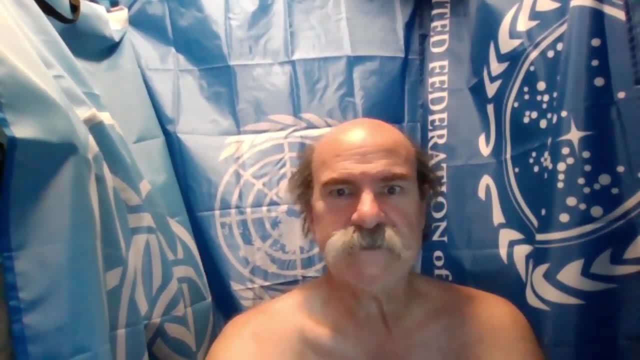 If one prisoner confesses, betrays the other one, while the other prisoner remains silent, the one who confesses is rewarded with a reduced sentence, while the other receives a harsh punishment. If both prisoners confess, if they each betray each other, they both receive a somewhat harsh punishment. 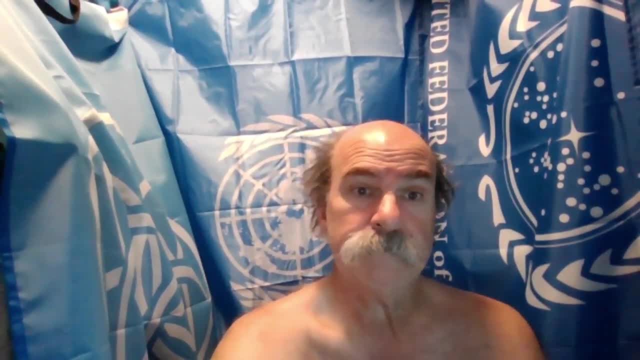 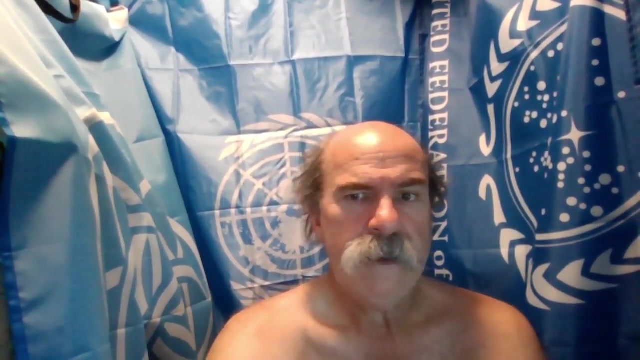 although less severe than if one prisoner had confessed. The dilemma arises from the conflict between individual incentives and the collective benefit of cooperation. From a self-interested perspective, each prisoner has an incentive to betray their partner, as it can lead to a reduced sentence or even avoiding punishment altogether. 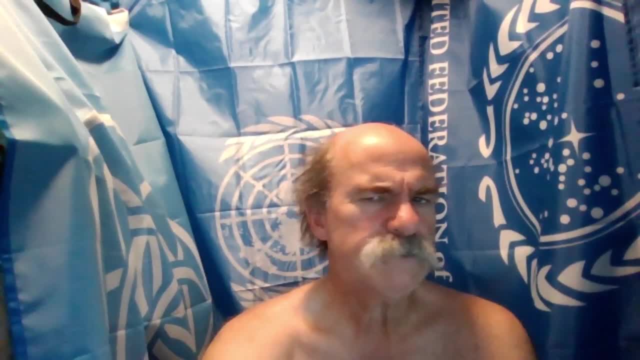 if the partner remains silent. However, if both prisoners betray, they both end up with a worse outcome compared to if they had both cooperated. The Prisoner's Dilemma highlights the tension between individual rationality and collective rationality, While it may seem rational for each prisoner, 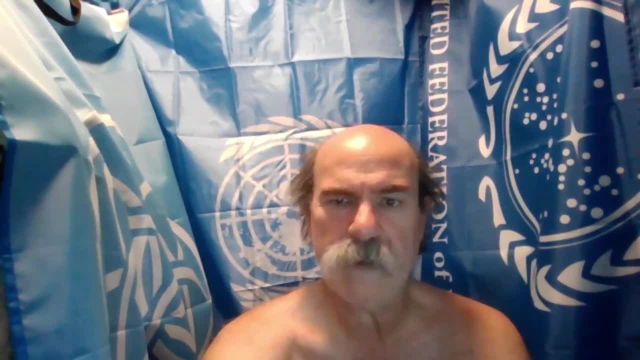 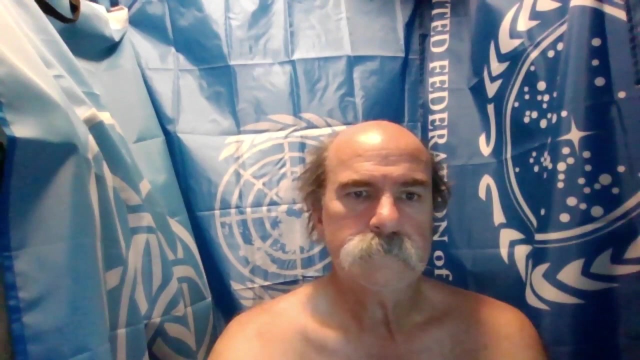 to betray. the collective outcome would be better if they both cooperated. The dilemma raises questions about trust, cooperation and the challenges of achieving mutually beneficial outcomes when individuals act solely in their own self-interest. The Prisoner's Dilemma serves as a powerful illustration. 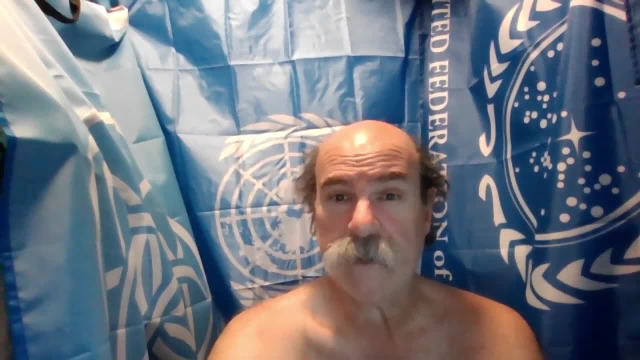 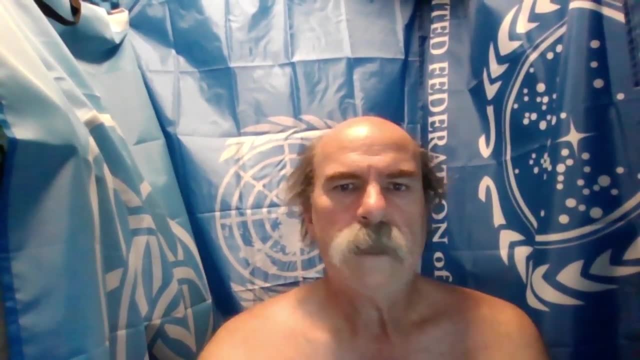 of the complexities of strategic decision-making and the challenges of cooperation and trust in competitive situations. The Battle of the Sexes scenario explores situations where individuals have different preferences or goals and must coordinate their actions to achieve the best possible outcome. It often represents a scenario where a couple must decide. 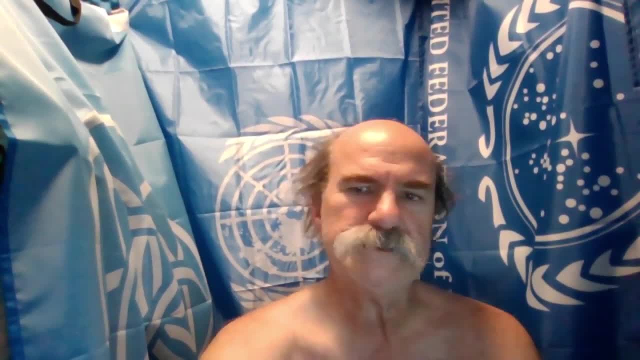 on an activity for the evening, but they have different preferences. For example, one person prefers going to a football game, while the other prefers going to the theater. In the Battle of the Sexes, there are typically two pure strategy equilibria. 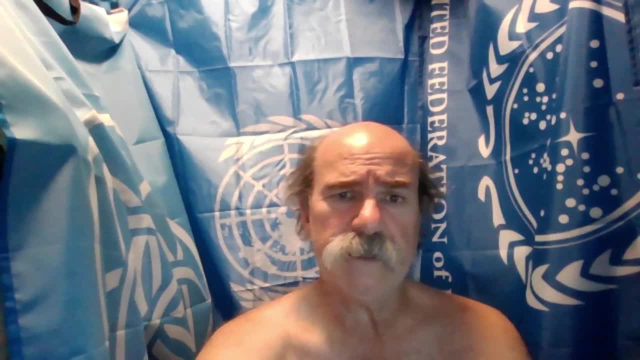 In the football equilibrium, both individuals choose to attend the football game. This outcome is preferred by one and is considered the best outcome for that individual. The other person may not be as satisfied, but they still prefer going to the football game over the theater. 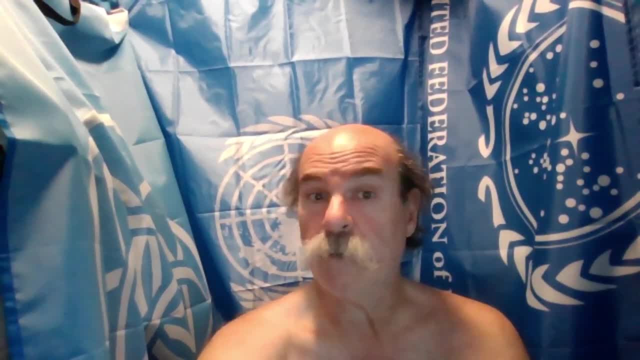 In the theater equilibrium. both individuals choose to go to the theater. Similarly, this outcome is preferred by one person and is considered the best outcome for that individual. The other person may not be as content, but they still prefer going to the theater over going to the football game. 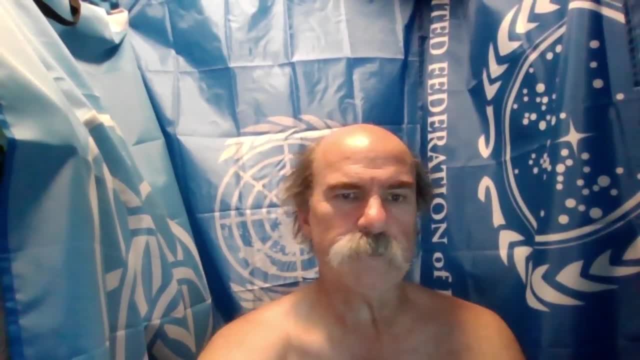 However, there is also a mixed strategy equilibrium. In the mixed strategy equilibrium, each person randomly chooses between the football game and the theater with a certain probability. For example, one person may choose the football game 60% of the time and the theater 40% of the time. 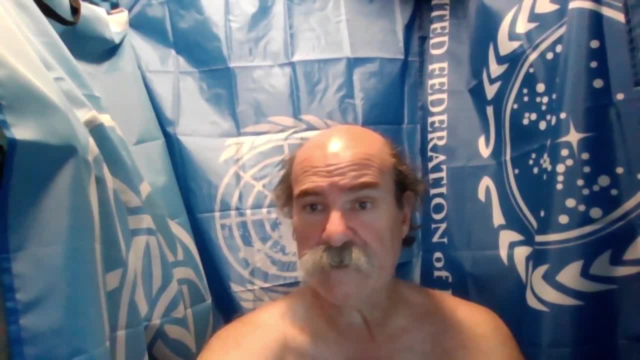 while the other person may choose the theater 60% of the time and the football game 40% of the time. This equilibrium arises when the individual's preferences are relatively balanced or when they wish to avoid conflict by compromising The Battle of the Sexes scenario. 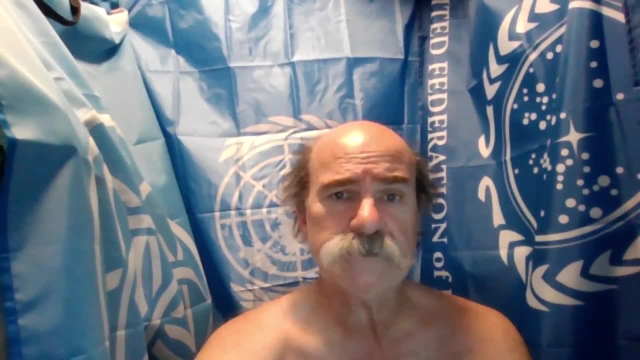 raises questions about coordination, communication and the challenges of finding a mutually satisfactory outcome when individuals have different preferences or goals. It highlights the importance of understanding each other's preferences, compromising or finding ways to coordinate actions to achieve a collectively desirable outcome. The Battle of the Sexes scenario. 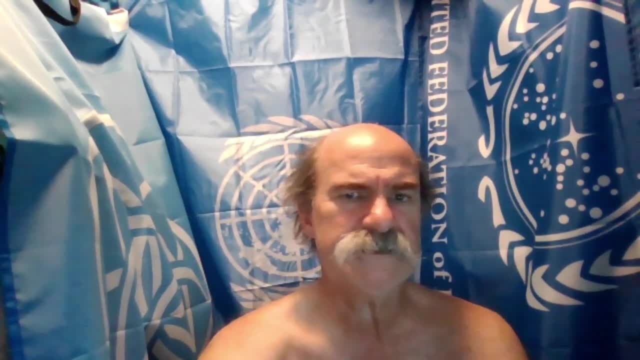 provides valuable insights into the complexities of decision-making in situations where individual preferences may not align perfectly. By studying this classic game theory scenario, we gain better understanding of the dynamics of coordination, compromise and the delicate balance between individual preferences and collective outcomes. The Chicken Game. 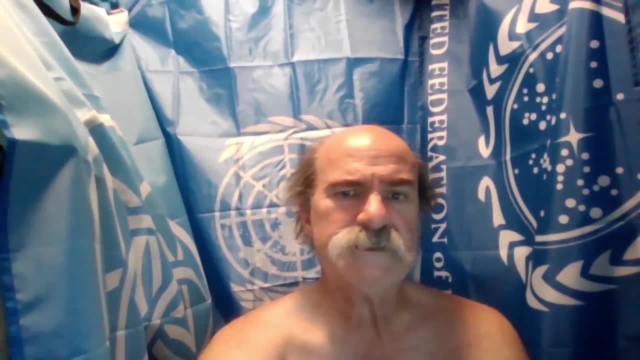 also known as the Hawk-Dove Game, represents a scenario where two players engage in a risky confrontation. It captures the tension between the desire to win and the potential cost of a dangerous outcome. In the Chicken Game, each player has to choose to either escalate the conflict. or swerve and avoid the confrontation. The outcomes of the Chicken Game can be represented as follows: If both players choose to escalate, they end up in a high-risk collision, resulting in a suboptimal outcome for both If one player escalates while the other player swerves. 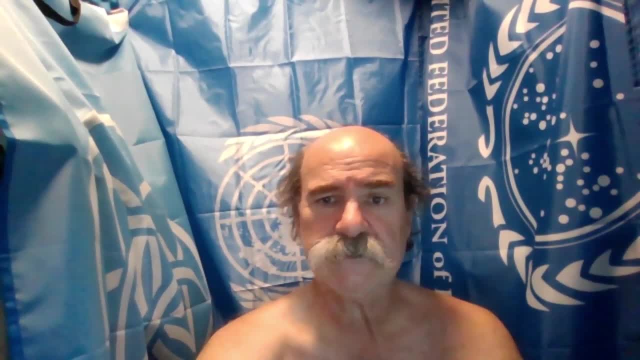 the player who escalates is considered more courageous and wins the confrontation, while the player who swerves is seen as weaker and less committed. If both players choose to swerve, they avoid the dangerous outcome and achieve a safer, though less exciting, outcome. 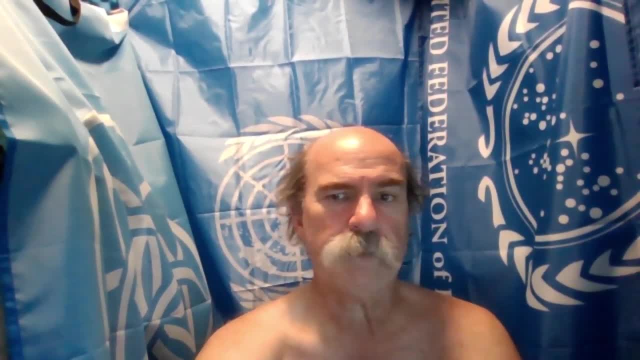 This outcome may be preferable when both players value safety and avoiding unnecessary risk. The Chicken Game highlights the trade-offs between the desire to win and the potential consequences of a dangerous outcome. It illustrates the dynamics of strategic behavior in situations involving risk and the delicate balance between courage and compromise. 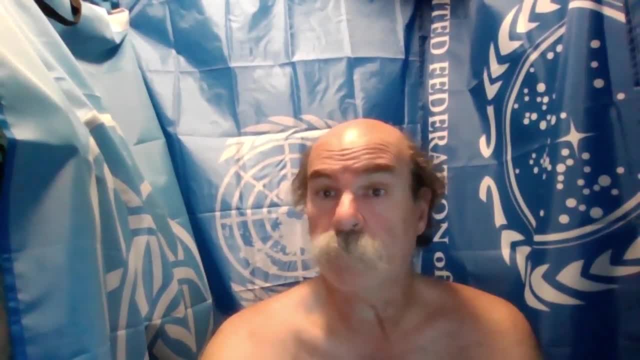 The Chicken Game can also be seen as a metaphor for various real-life scenarios, such as political negotiations, economic competitions or personal relationships. It raises questions about decision-making under risk, the psychology of bluffing and the dynamics of brinkmanship. The Chicken Game provides valuable insights. 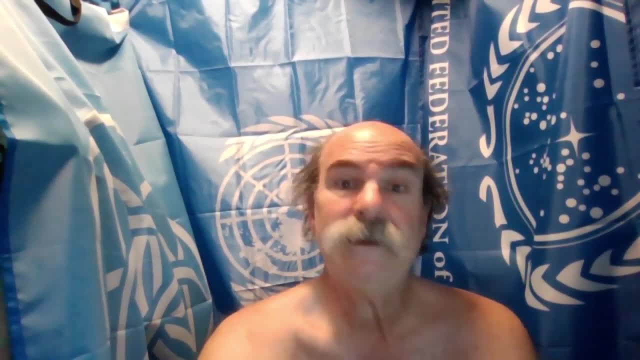 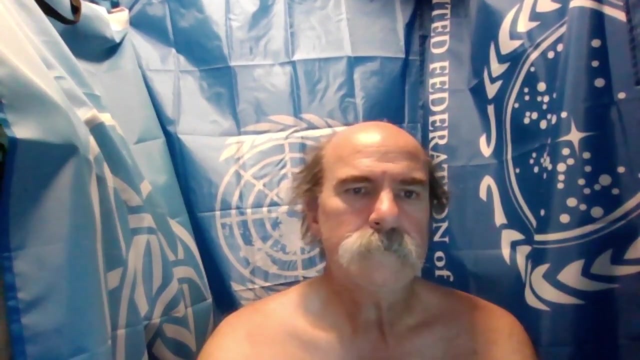 into the complexities of strategic behavior, strategic decision-making in high-stakes situations. By studying this classic game theory scenario, we gain a deeper understanding of the challenges involved in balancing risk, courage and the pursuit of favorable outcomes, As we have seen. 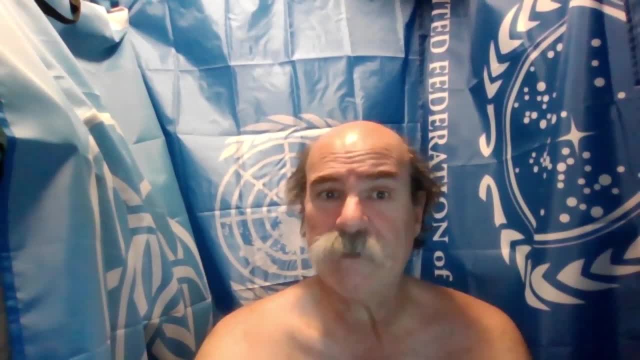 the Chicken Game offers valuable insights into the dynamics of strategic decision-making under risk and the delicate balance between courage and compromise. By studying this classic scenario, we gain a better understanding of the complexities of bluffing, risk assessment and the pursuit of optimal outcomes. 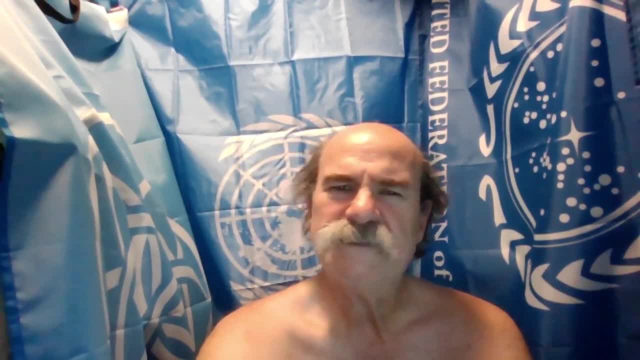 in competitive situations. The Stag Hunt scenario explores the dynamics of cooperation and coordination in a strategic interaction. In this scenario, two hunters must decide whether to cooperate and hunt the stag, which provides a larger reward, or act individually and hunt a smaller game. 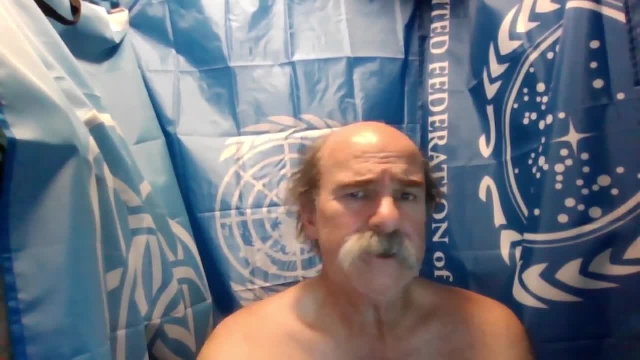 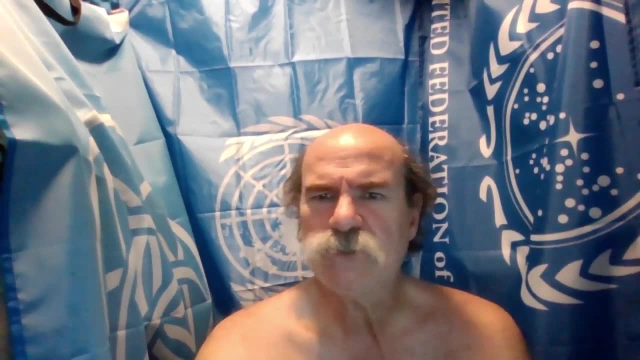 such as a hare. The Stag Hunt scenario highlights the tension between individual incentives and collective benefits. If both hunters choose to cooperate and hunt the stag, they can secure a higher payoff together. However, there is risk involved If one hunter chooses to hunt the stag. 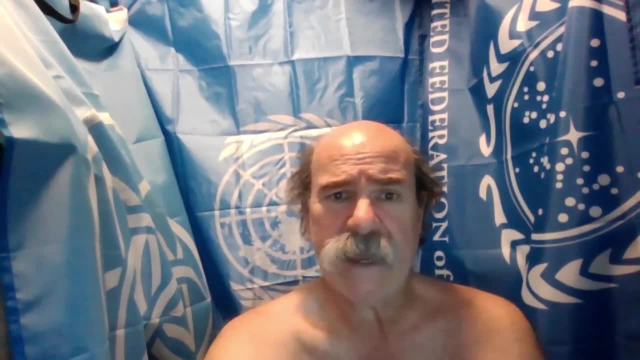 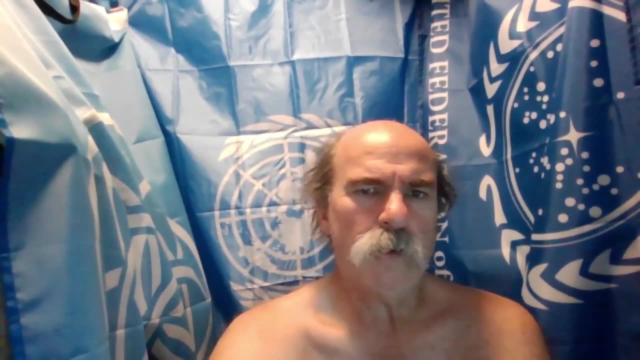 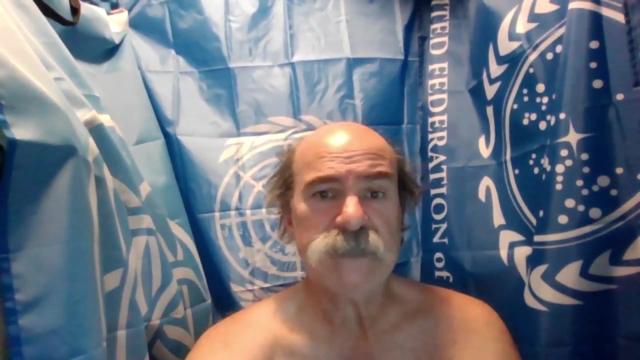 while the other hunts a hare, the hunter pursuing the stag risks ending up empty-handed if the other hunter fails to cooperate. The Stag Hunt scenario offers multiple, multiple equilibrium. In the stag equilibrium, both hunters coordinate their actions and choose to hunt the stag. 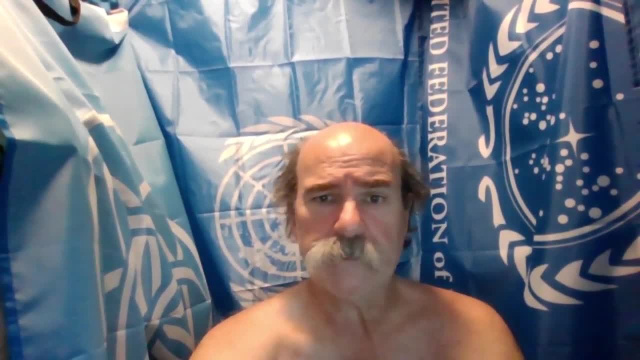 The outcomes yield the highest payoff for both hunters. However, reaching this equilibrium requires trust, communication and a shared understanding that both hunters will cooperate In the hare equilibrium. both hunters independently choose to hunt the hare, opting for the safer option with a guaranteed payoff. 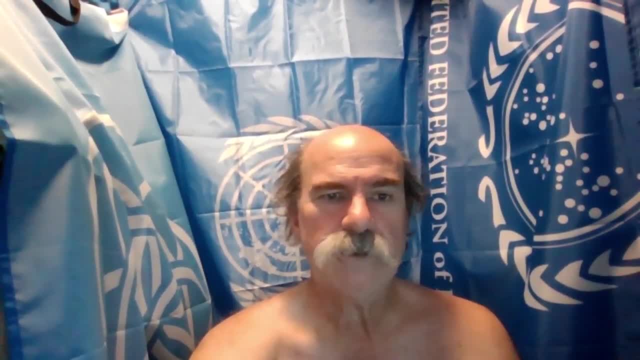 This outcome may arise when there is lack of trust or hunters prioritize their individual interests over the potential higher payoff of hunting the stag. The Stag Hunt scenario raises questions about trust, communication and the challenges of achieving cooperation and coordination in situations where individual incentives 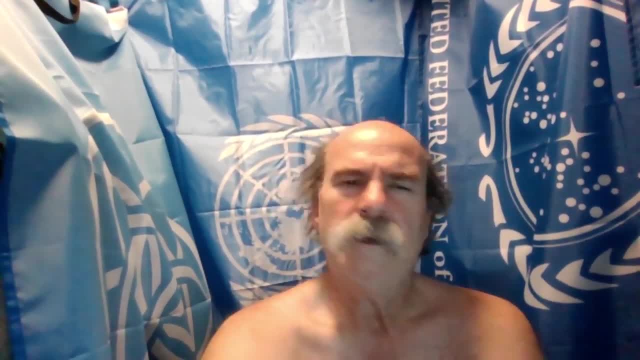 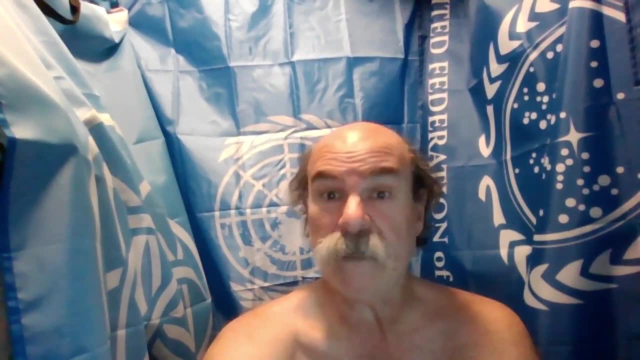 may conflict with collective benefits. It underscores the importance of aligning interests, establishing trust and effectively communicating to achieve the best possible outcome for all participants. The Stag Hunt scenario provides valuable insights into the complexities of cooperation and coordination in strategic interactions By studying this classic game theory scenario. 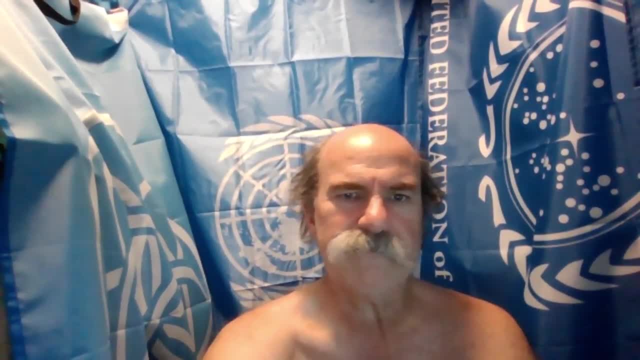 we gain deeper understanding of the challenges involved in achieving collective success and the delicate balance between individual actions and the overall outcome. The Chicken and the Egg scenario explores a unique situation where the order of actions or events is crucial. It represents a scenario where two players must make a decision. 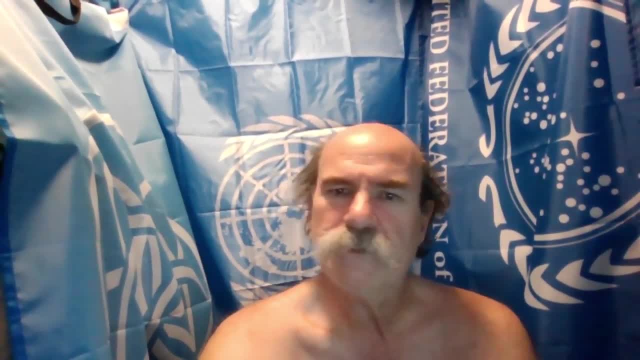 without knowing the other player's choice, but their choices are interdependent and can lead to different outcomes based on the order of actions. In the Chicken and Egg scenario, the outcomes depend on who takes the initiative If both players wait for the other to take action. 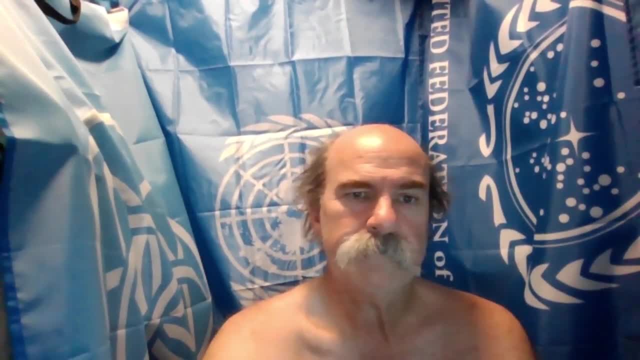 they end up in a stalemate, unable to progress. If one player takes the initiative and makes a move, it can influence the other player's decision. The player who acts first gains an advantage in shaping the outcome If both players take simultaneous actions. 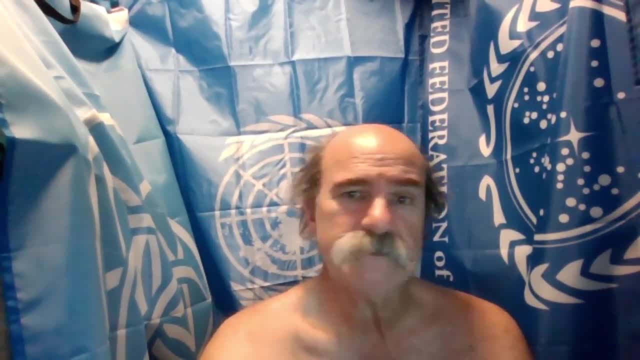 the outcome depends on the compatibility of their choices. If their actions are aligned and complementary, it can lead to a favorable outcome for both. However, if their choices conflict, it can lead to a suboptimal or conflicting outcome. The Chicken and Egg scenario. 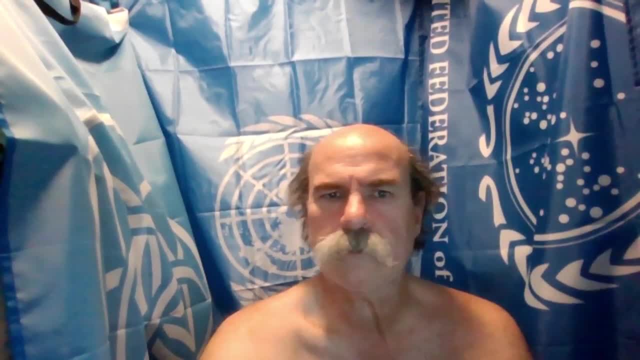 highlights the importance of timing initiative and the interplay between individual decisions and their impact on the overall outcome. It raises questions about strategic sequencing, the psychology of waiting and the challenges of making choices without complete information. The Chicken and Egg scenario provides valuable insights. 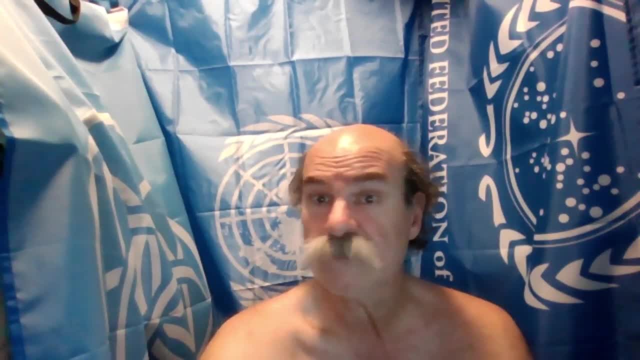 into the complexities of decision making when the order of actions is crucial. By studying this unique game theory scenario, we gain a deeper understanding of the challenges involved in timing, initiative and the delicate balance between individual decisions and their influence on collective outcome. 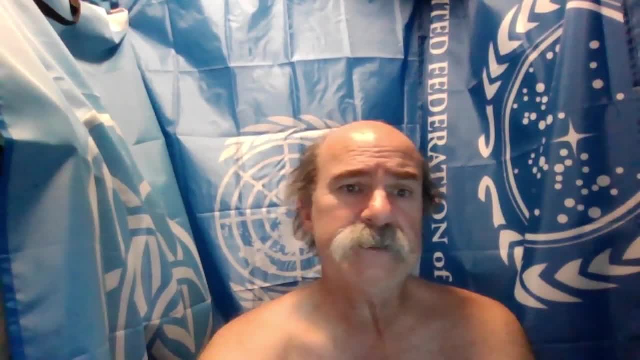 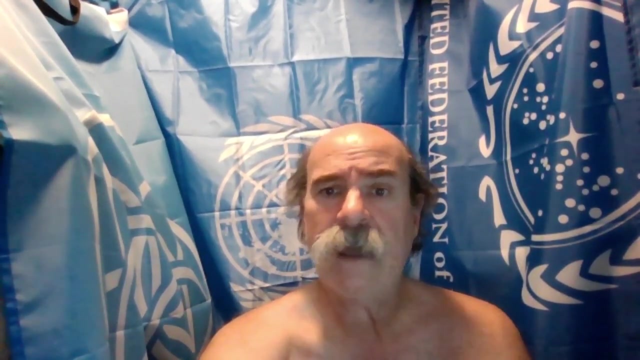 As we have seen, the Chicken and Egg scenario offers valuable insights into the dynamics of decision making when the order of events or actions is critical. By studying this classic scenario, we gain a better understanding of the complexities of timing, initiative and the pursuit of optimal outcomes. 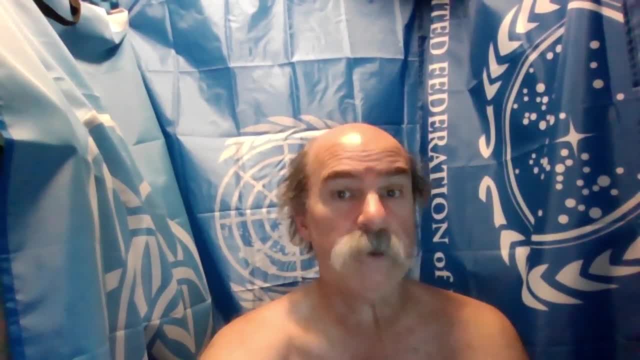 in situations where individual choices are interdependent. These classic game theory scenarios provide captivating insight into strategic decision making and the complexities of human behavior. They offer valuable lessons about cooperation, trust, risk coordination and the delicate balance between individual and collective interests. 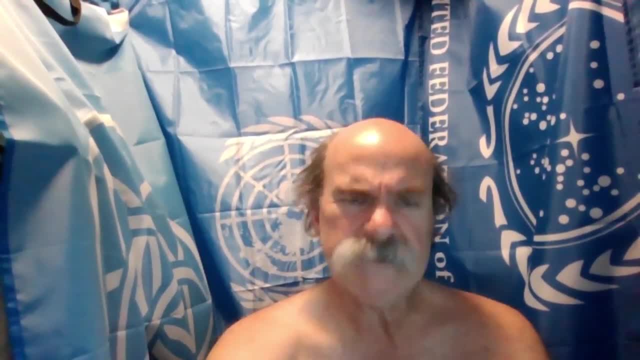 As we've explored the classic game theory scenarios, it's important to note that they represent simplified models that capture certain aspects of real-life situations. In a minute, we'll discuss the criticisms and limitations of game theory, acknowledging that real-world scenarios are often more complex and nuanced. 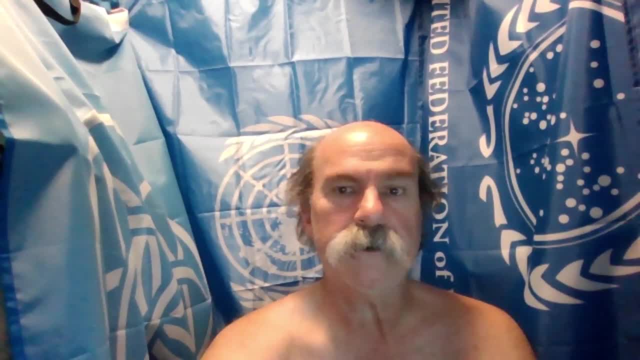 By studying classic game theory scenarios, we can gain valuable insights into strategic interactions and decision making. However, it's essential to remember that these scenarios serve as abstractions and simplifications of real-life situations. Now that we've explored the fundamental concepts of game theory, 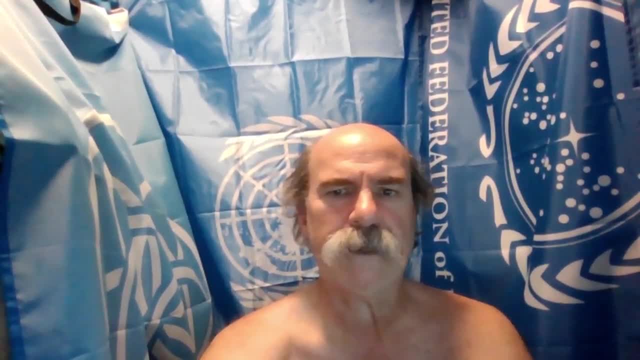 let's turn our attention to real-world applications and implications of this powerful framework. Game theory has made significant contributions to economics by providing insights into strategic interactions and insights into strategic behavior, market dynamics and decision making in various economic contexts. It helps economists analyze competition. 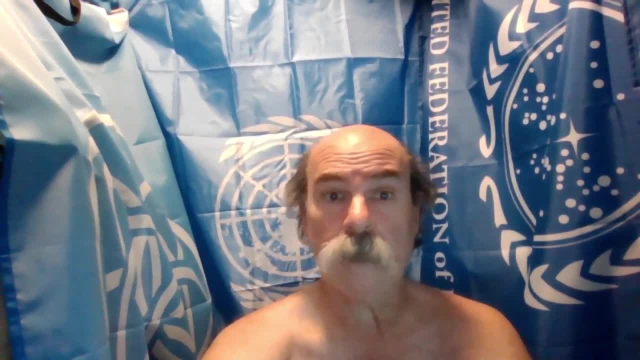 pricing strategies, oligopolies, auctions and negotiations. Game theory also plays a crucial role in understanding market failures, designing mechanisms for resource allocation and studying the impact of regulations and policy interventions. Game theory has practical applications in business strategy and competitive analysis. 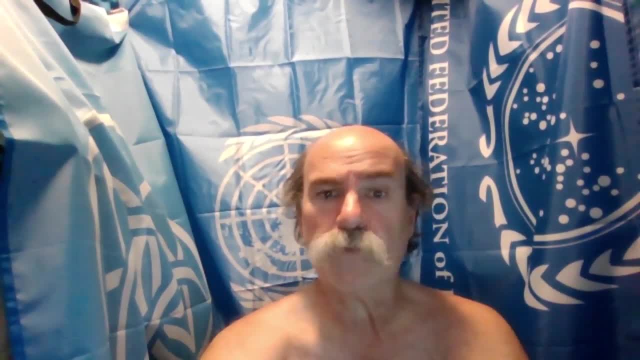 It helps companies make informed decisions about pricing, product differentiation, market entry and advertising. By applying game theory models, businesses can analyze rivalries, strategic interactions and optimal decision making strategies. Game theory also guides negotiations, strategic alliances and the formulation. 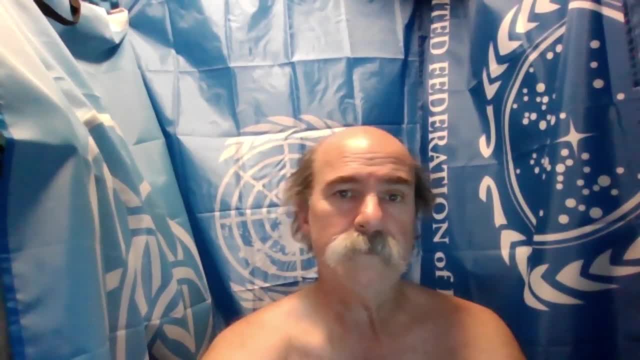 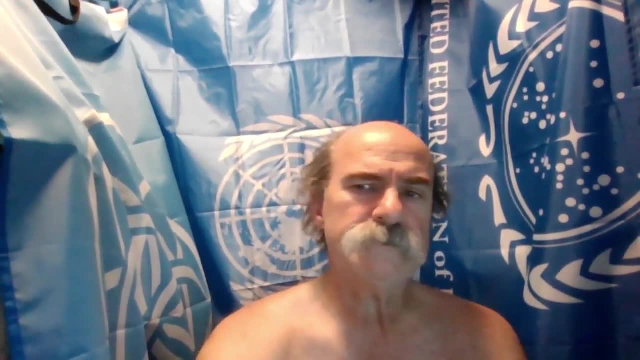 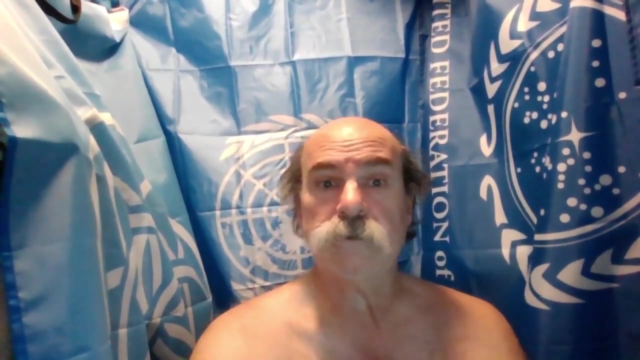 of optimal bidding strategies and auctions. Game theory provides valuable insights into political behavior, international relations and voting systems. It helps analyze strategic decision making in elections, coalition formations and policy negotiations. Game theory models shed light on arms races, conflicts and the dynamics of cooperation. 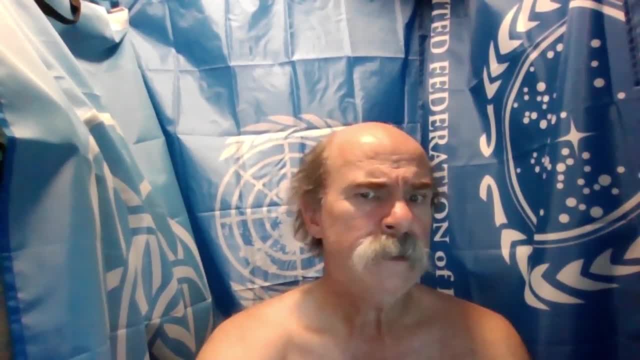 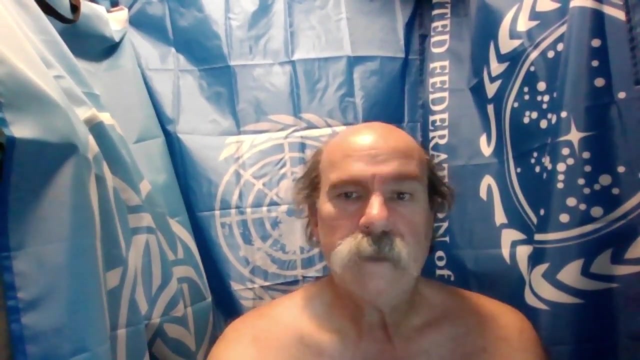 and defection between nations. It assists policymakers in understanding the incentives and outcomes of different policy choices. Game theory has found applications in studying the dynamics of biological systems and evolution. It helps analyze interactions among species, mating behaviors, predator-prey relationships and the evolution 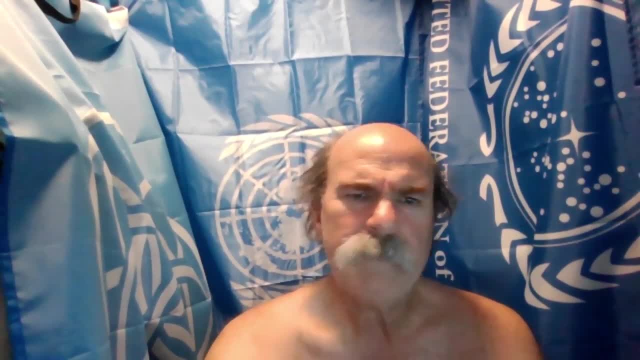 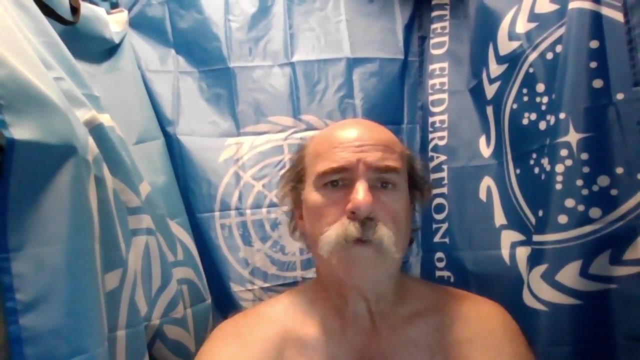 of cooperative behaviors. Game theory models shed light on the development of social norms, altruistic behaviors and the emergence of stable strategies in evolving populations. Game theory is also relevant in social sciences, where it provides insight into human behavior, social interactions and decision making. 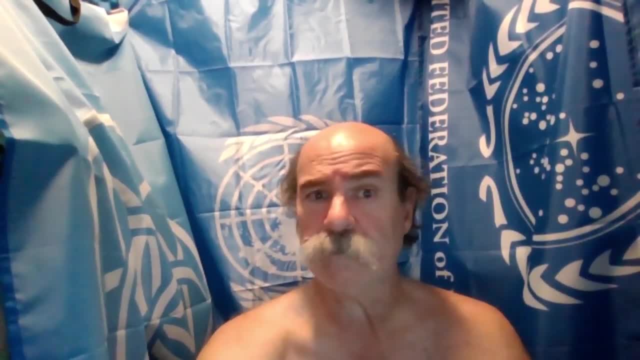 It helps understand cooperation, trust and conflict resolution in social dilemmas. Game theory is applied in fields such as sociology, psychology, anthropology and behavioral economics to examine decision making processes, social norms and collective actions. Game theory is an integral part. 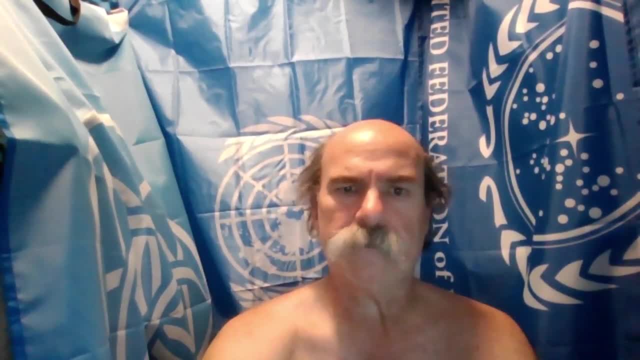 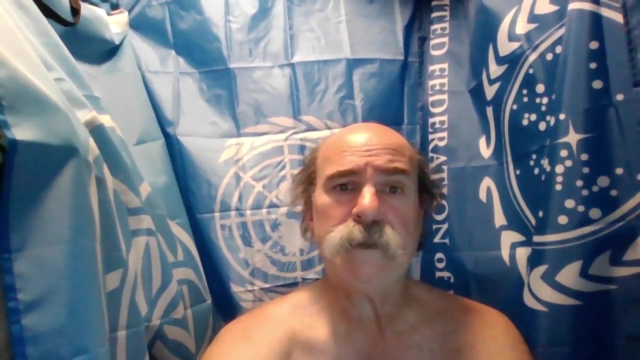 of developing intelligent systems and algorithms in artificial intelligence. It helps design strategic decision making agents, predict opponent behavior and optimize outcomes in multi-agent environments. Game theory provides a foundation for developing algorithms in areas such as automated negotiation, auction design and multi-agent coordination. 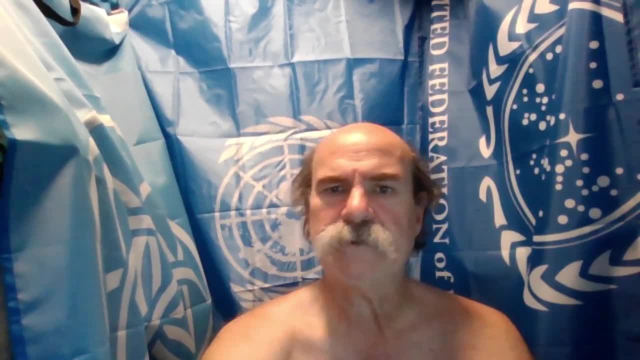 Game theory's applications span diverse fields, including economics, business strategy, political science, biology, social sciences and artificial intelligence. By providing a framework to analyze strategic interactions, game theory equips us with tools to make informed decisions, predict outcomes and optimize strategies. 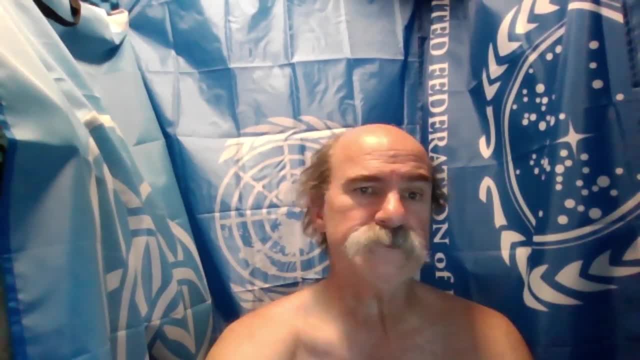 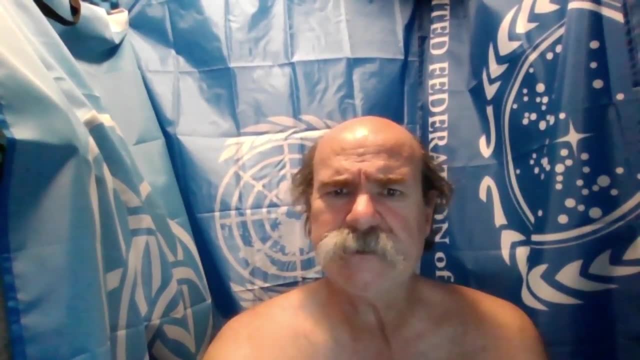 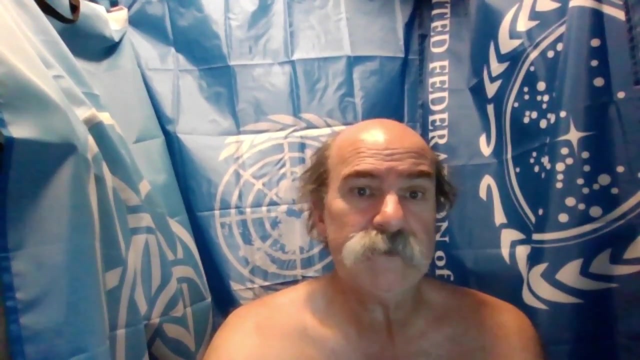 in a wide range of real-world scenarios. Game theory offers valuable insights into decision making, strategic interactions and the complexities of human behavior. By exploring its applications and implications, we can better understand the dynamics of competitive environments, cooperation, conflict resolution and the pursuit. 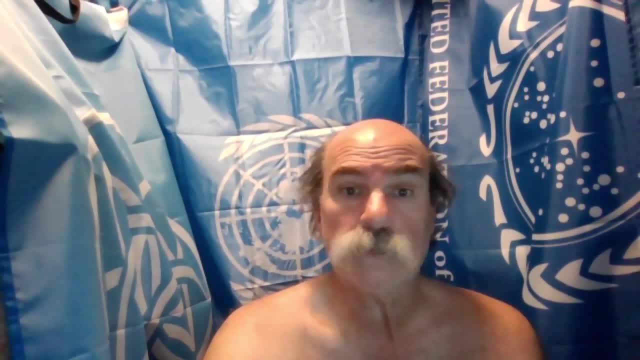 of individual and collective goals. Game theory finds practical applications in numerous fields, offering valuable insights into decision making, strategic interactions and optimal strategies. Game theory provides practical applications in numerous fields, offering valuable insights into decision making, strategic interactions and optimal strategies. 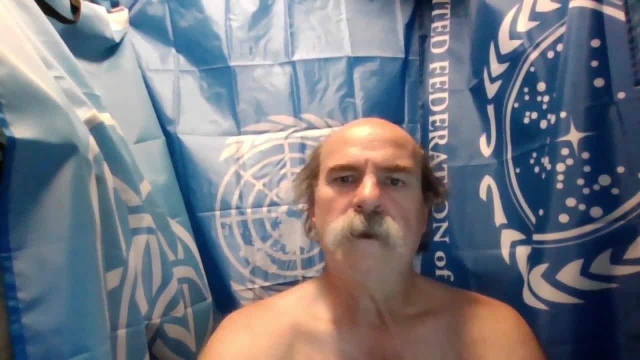 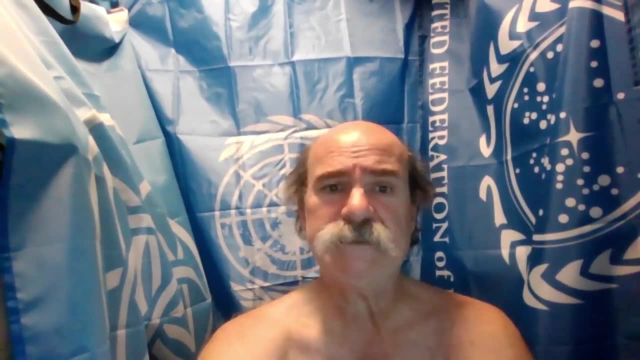 Let's delve into some real-life applications of game theory. Game theory plays a significant role in economics and finance. It helps analyze market competition, pricing strategies and the dynamics of oligopolies. Game theory models are used to study auctions bargaining. 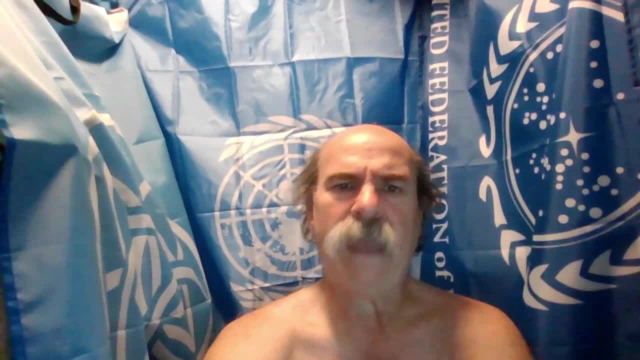 and negotiation strategies In finance. game theory aids in understanding investor behavior, portfolio management and pricing of complex financial instruments. Game theory provides insights into strategic decision making in business and marketing. Companies use game theory to analyze pricing strategies, product differentiation and market entry decisions. 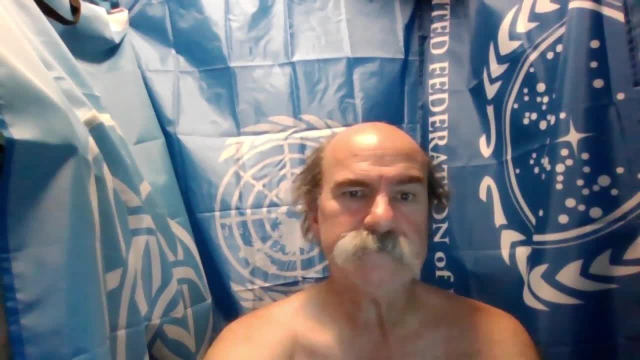 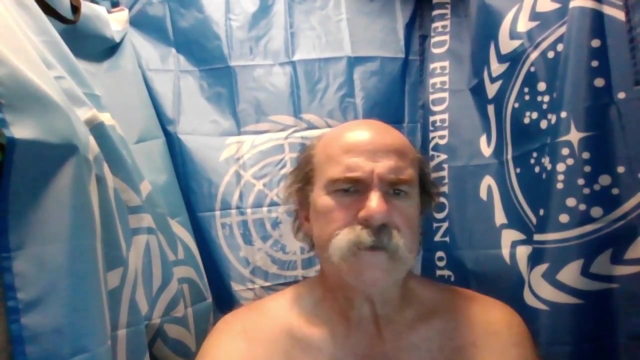 It assists in understanding competitive dynamics, advertising campaigns and brand positioning. Game theory models are also employed in supply chain management, inventory control and strategy management. Game theory models are used to analyze the market's market and strategic alliances. Game theory has practical applications. 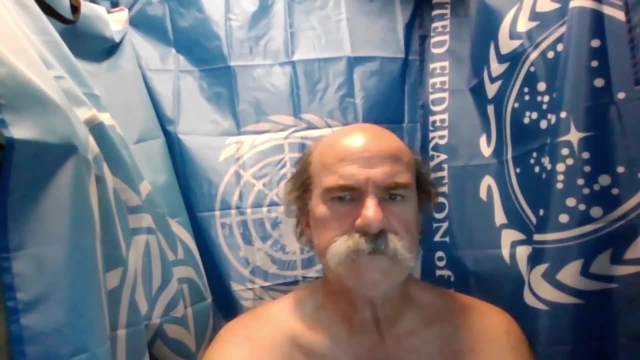 in political science and international relations. It helps analyze strategic interactions between political actors, negotiation processes and coalition formations. Game theory models shed light on voting systems, electoral campaigns and policy decision making In international relations. it helps understand conflicts, arms races. 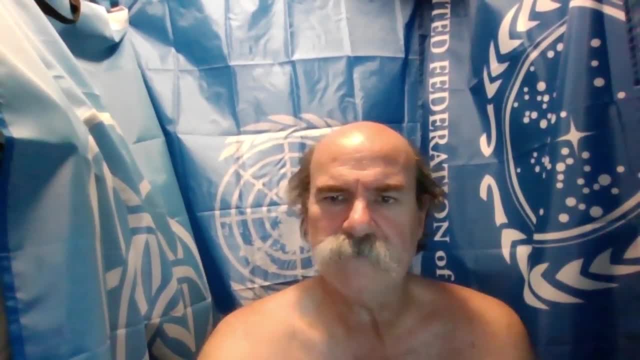 and negotiation between countries. Game theory models shed light on political science and international relations. Game theory is applied in environmental science and resource management to analyze the strategic interactions related to resource allocation, pollution control and conservation efforts. It aids in understanding cooperation agreements such as: 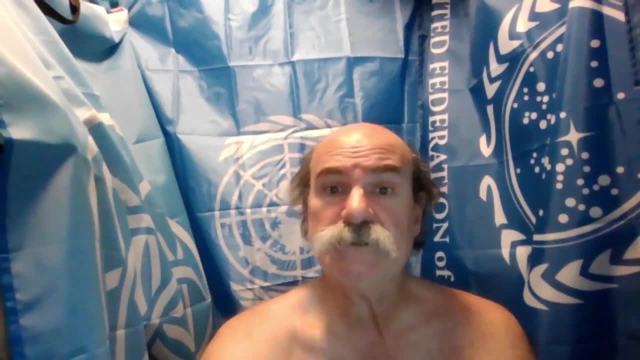 international climate change negotiations and the design of mechanisms for sustainable resource management. Game theory plays a role in understanding social networks and online platforms. Game theory plays a role in understanding social networks and online platforms. It helps to analyze user behavior. strategies for viral marketing. 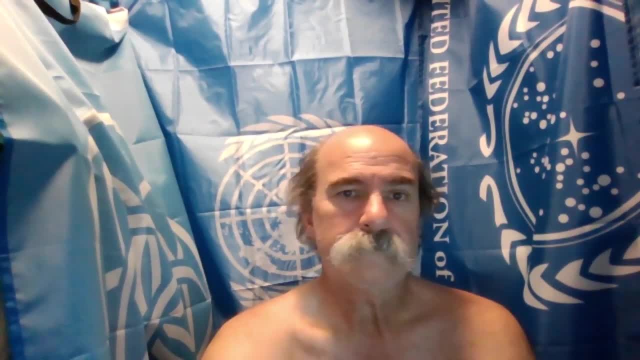 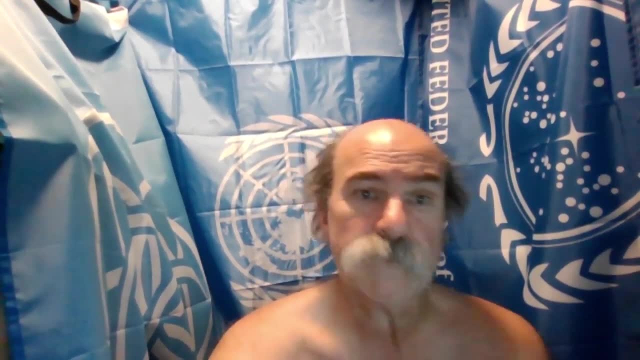 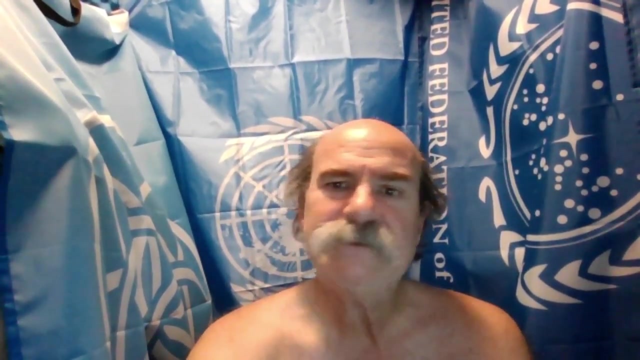 and the dynamics of network effects. Game theory models assist in designing incentive mechanisms, reputation systems and algorithms for personalized recommendations. Game theory finds applications in healthcare and epidemiology. It aids in analyzing the spread of infectious diseases, vaccination strategies and the dynamics. 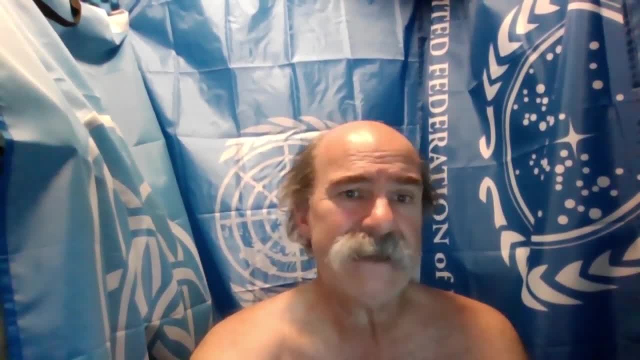 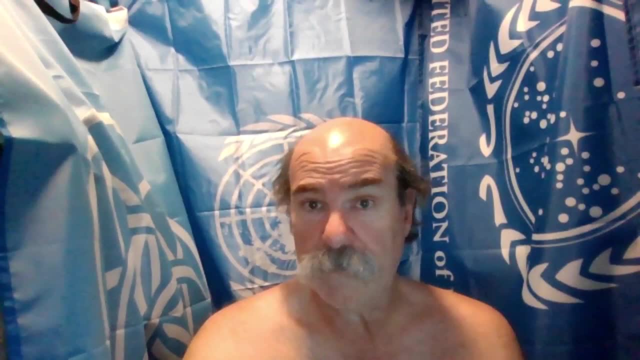 of herd immunity. Game theory finds applications in healthcare and epidemiology. Game theory models assist in studying the strategic interaction among healthcare providers, resource allocation in healthcare systems and the impact of public health interventions. Game theory provides insights in the legal contexts and negotiation. 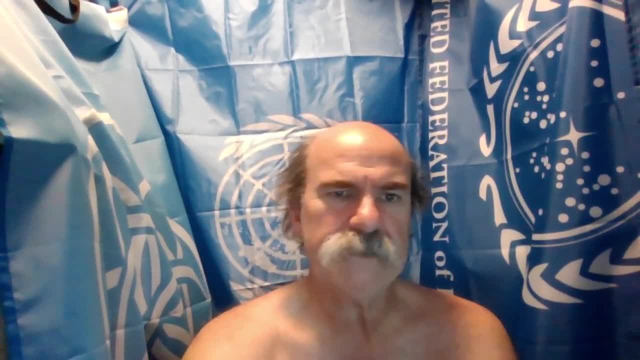 strategies. It helps analyze settlement negotiations, plea bargaining and strategic behavior in legal disputes. Game theory models assist in understanding the dynamics of contract negotiations, intellectual property disputes and the design of legal frameworks. Game theory is an integral part of developing intelligent systems. 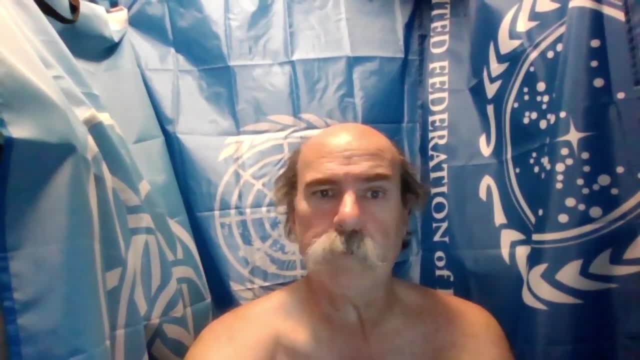 and algorithms in artificial intelligence and robotics. It helps design autonomous agents, multi-agent systems and algorithms for decision making under uncertainty. Game theory models are used in automated negotiation, robot coordination and algorithmic mechanism design. These are just a few examples of how game 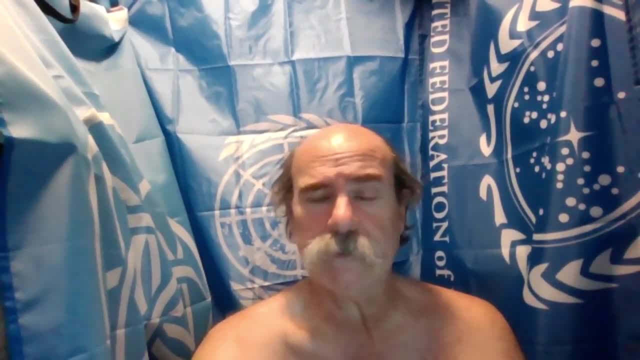 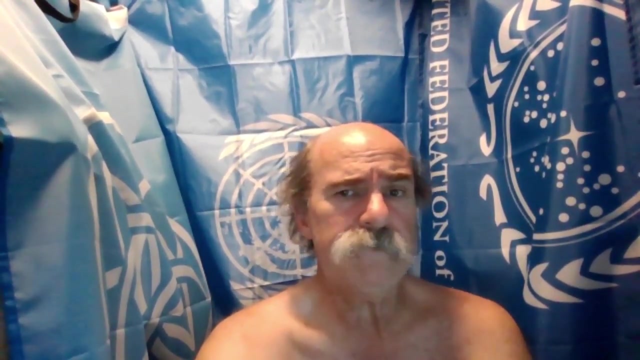 theory is applied in real life situations across various fields. By employing game theory models, practitioners can gain insights into strategic decision making, predict outcomes and optimize strategies for improved results. Game theory continues to evolve and find new applications as we encounter complex challenges in our ever-changing. 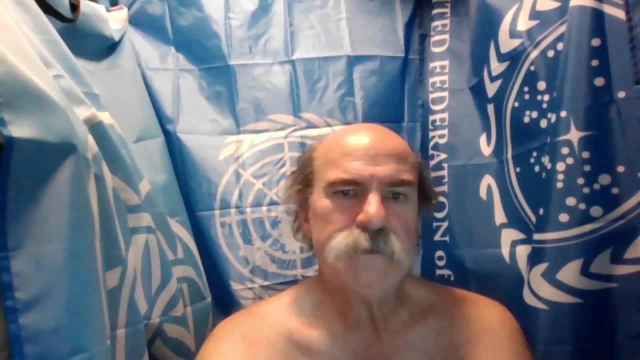 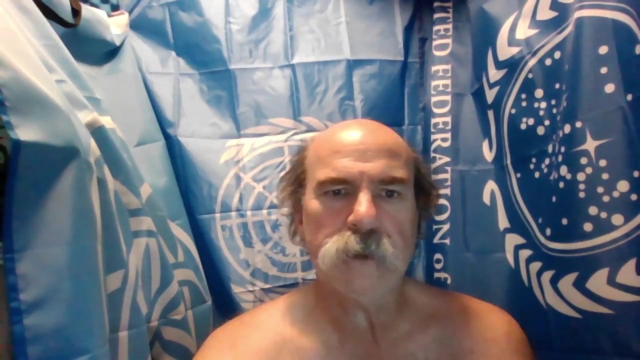 world. Its practical implications help us navigate competitive environments, design efficient systems and make informed decisions in a wide range of real-life scenarios. In game theory, we often encounter scenarios where cooperation among players can lead to mutually beneficial outcomes. This brings us to the realm. 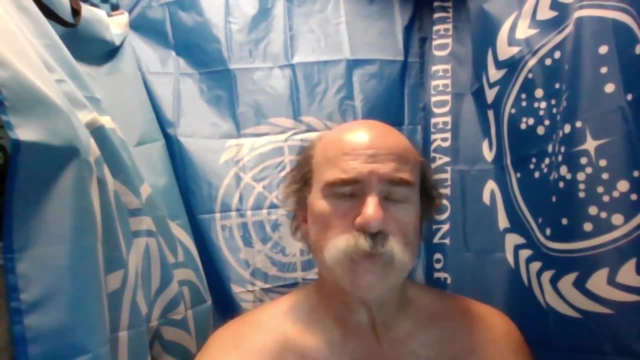 of cooperative game theory, which explores situations where players can form coalitions and work together to achieve favorable results. Let's delve into this fascinating aspect of game theory. In cooperative game theory, the focus shifts from individual decision making to group interactions. Players can 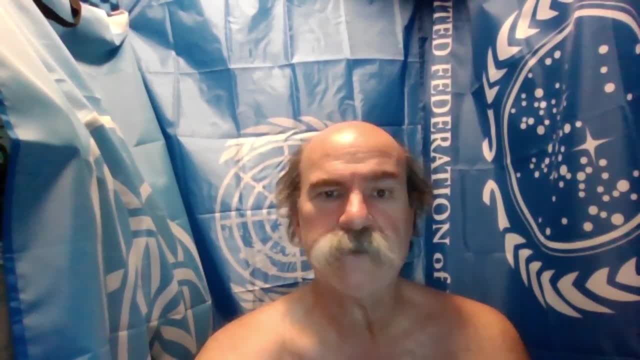 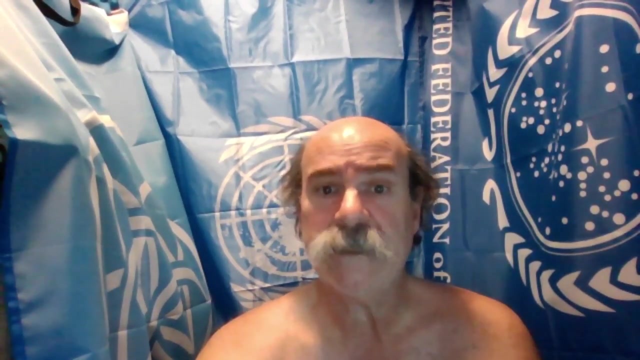 form coalitions, which are groups of players who collaborate to achieve common objectives. These coalitions may have varying degrees of stability and power dynamics. Cooperative games are characterized by a characteristic function which assigns a value or utility to each possible coalition. This function- 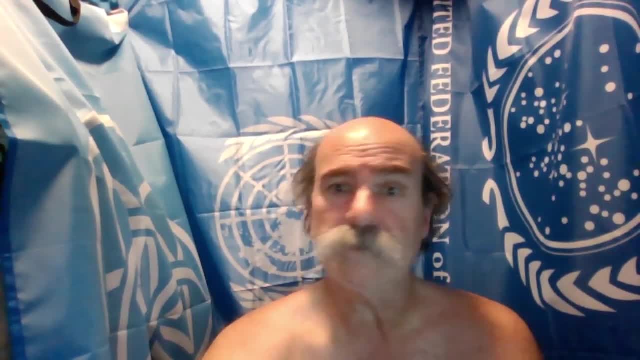 represents the benefits that the coalition can generate collectively. Additionally, cooperative games often assume transferable utility, meaning that the total payoff or value generated can be divided among the players. Cooperative game theory introduces solution concepts that allocate the collective benefits among the players in a fair 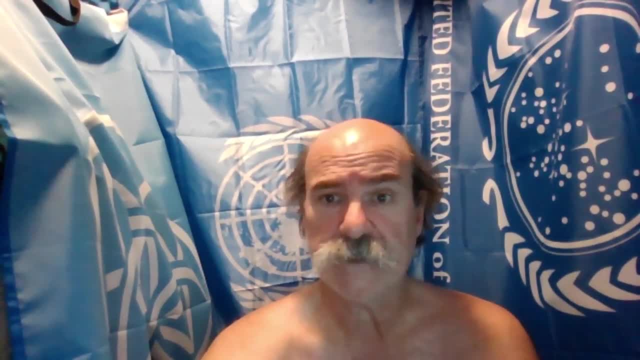 and efficient manner. One popular solution concept is the concept of a coalition's worth or shapely value, which distributes the value generated by the coalition among its players based on their contributions. Other solution concepts include the nucleus, the core and the bargaining. set, each with its own approach to distributing the gains. Cooperative game theory finds applications in various fields. In economics, it helps analyze cooperative production, joint ventures and resource allocation in collaborative settings. In politics, it aids in understanding coalition formations, power sharing. 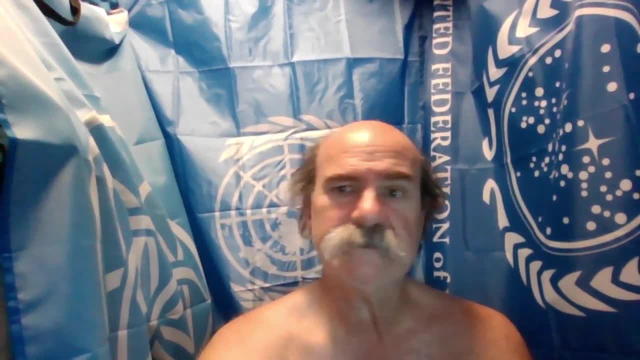 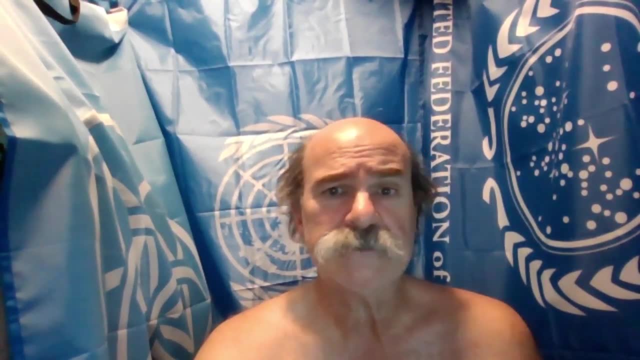 arrangements and the distribution of benefits and alliances. Cooperative game theory is also applied in the analysis of collaborative decision making in areas such as climate change agreements, international negotiations and public policy formation. While cooperative game theory offers valuable insights into collective decision making, 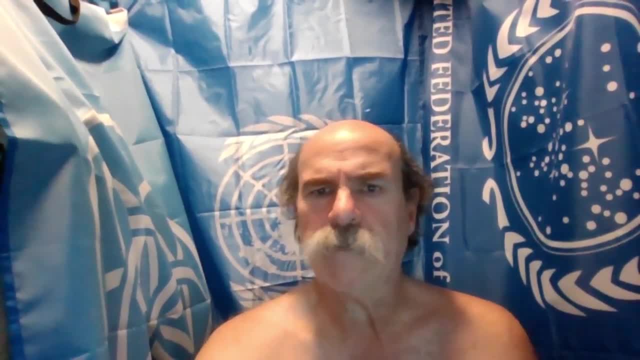 it also presents challenges. Determining fair allocations and accounting for players' contributions can be complex, especially in large-scale cooperative games. Additionally, the stability and sustainability of coalitions and the potential of free-riding or shirking within coalitions are important. considerations. Cooperative game theory expands our understanding beyond zero-sum games in competitive interactions, highlighting the potential for collaboration and mutual gains. By exploring cooperative game theory, we can identify ways to foster cooperation, negotiate fair agreements and achieve more possible outcomes in various domains. 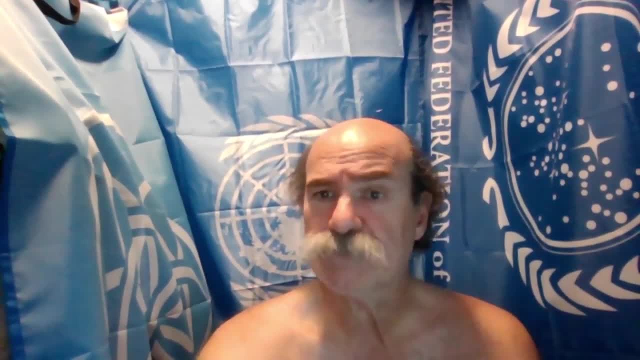 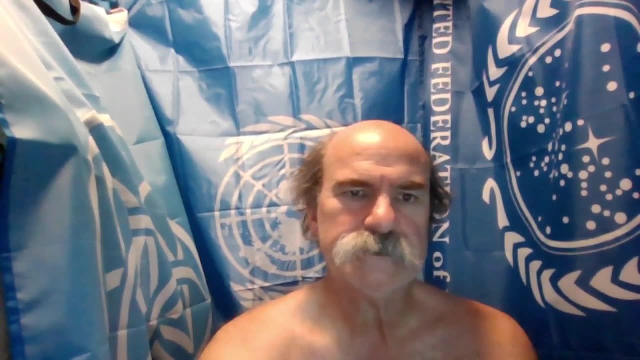 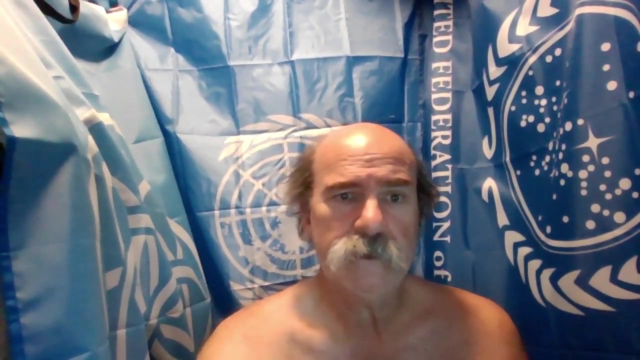 While game theory provides valuable insights into strategic decision making, it's not without its limitations and criticisms. Let's explore some of these concerns. Game theory often relies on simplifying instructions about players' rationality, perfect information and the ability to accurately assess. 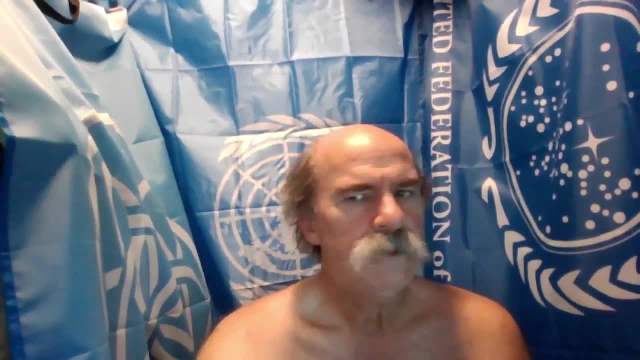 payoffs. In reality, human behavior can be more complex, influenced by emotions, biases and bounded rationality. Critics argue that game theory's assumptions may oversimplify real-world decision-making processes. Game theory assumes that players act rationally, striving to maximize 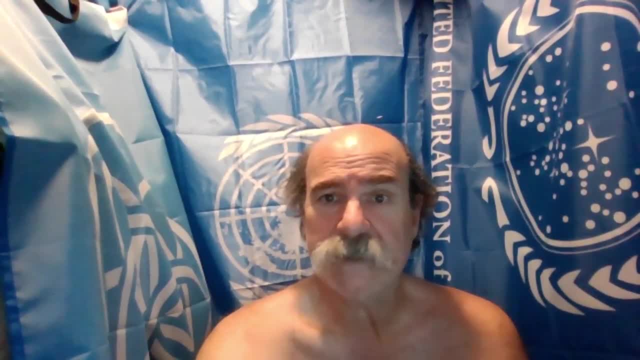 their payoffs. However, human behavior is not always predictable or purely rational. As a result, game theory assumes that players act rationally. Ask Mr Spock. Factors like social norms, cultural influences and psychological biases can impact decision-making. 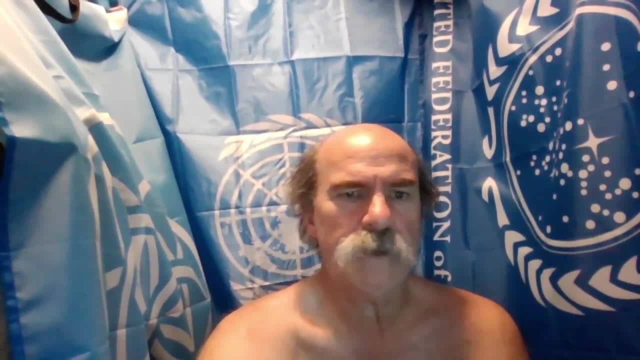 making it challenging to accurately predict how players will behave in strategic situations. Game theory focuses on individual interactions and strategies, often overlooking the broader context within which games are played. Critics argue that, considering contextual factors such as social structures, power dynamics and historical 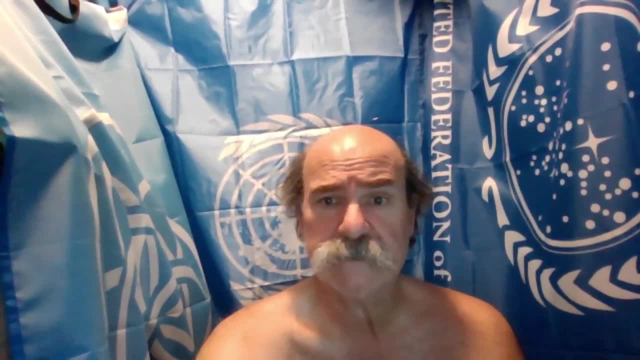 precedents is essential for a more comprehensive understanding of strategic decision making. Some critics raise ethical concerns about game theory's emphasis on strategic calculations and the potential for exploitation. They argue that solely focusing on achieving the best outcome for oneself or a specific group may 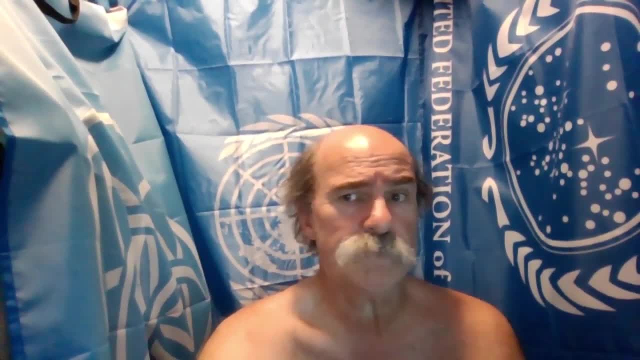 neglect broader ethical principles, fairness and considerations of societal values. Game theory is not the only example of game theory. While game theory has found success in certain simplified scenarios, its application becomes more challenging in complex real-world situations with multiple interrelated factors. 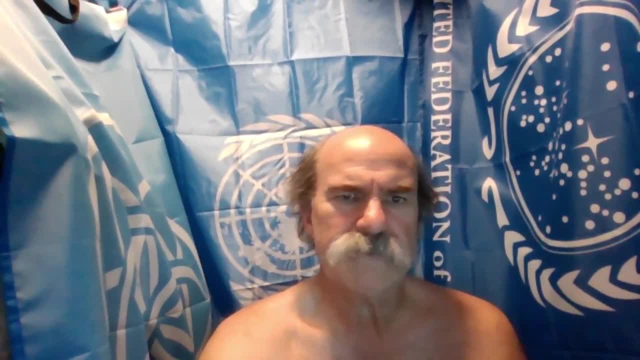 The practical implications of game theory models and predictions may face difficulties due to the dynamic nature of real-world environments. Game theory traditionally assumes that players act in their own self-interest, but it may not fully capture cooperative or altruistic behaviors that emerge in real-world settings. 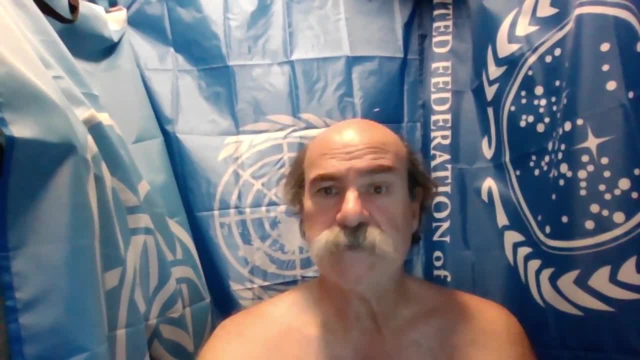 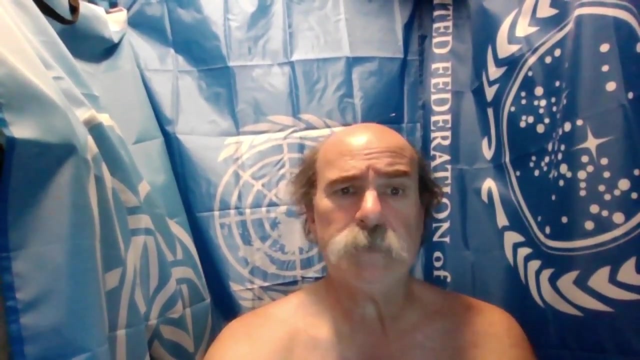 Understanding the conditions under which cooperation and altruism arise and how they influence strategic interactions remain an ongoing challenge in game theory. It's important to acknowledge the limitations and criticisms of game theory as we apply it to real-world scenarios. While it provides valuable insights, 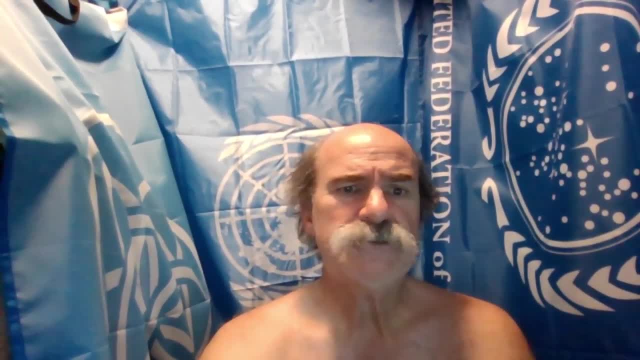 it should be used in conjunction with other analytical approaches. It should be used in collaboration with other analytical tools, empirical evidence and contextual considerations. By recognizing these limitations, we can continue to refine and develop game theory to better capture the complexities of decision-making. 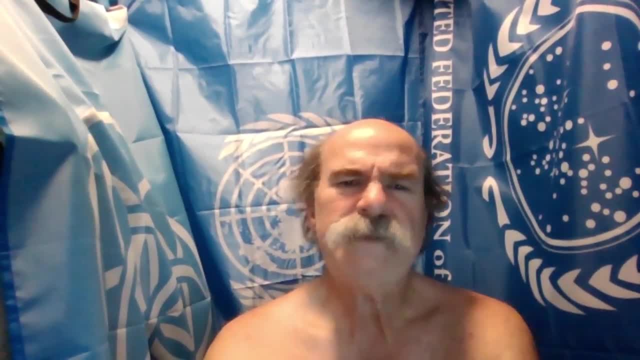 and strategic interactions in a diverse range of situations. Today, we've explored the fascinating world of game theory, from its foundational concepts to its real-life implications. Game theory offers valuable insights into strategic decision-making, the dynamics of competitive interactions and the complexities of 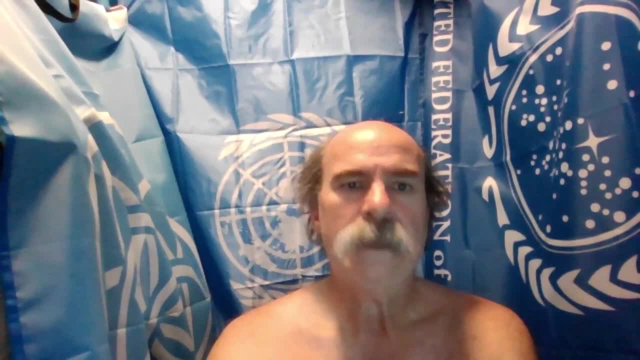 human behavior. Let's recap what we've learned. Game theory provides a framework for analyzing strategic situations where the outcomes of one's actions depend on the actions of others. It examines players, strategies, payoffs, information and game forms to understand. 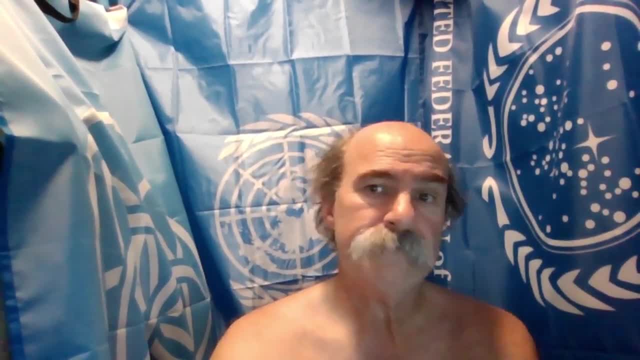 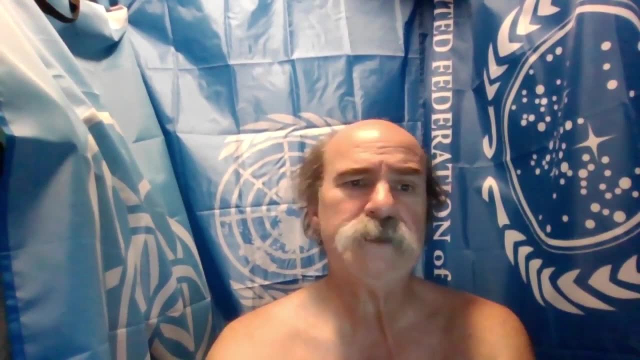 how rational actors make choices in various scenarios. Equilibrium concepts such as Nash Equilibrium and Dominant Strategy Equilibrium help us predict stable outcomes and optimal strategies. We have seen how game theory is applied in economics, business strategy, political science, biology. 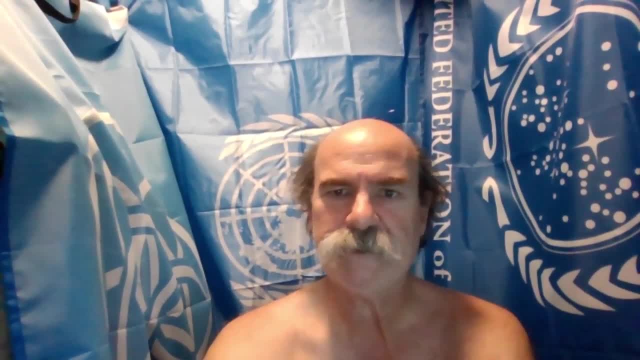 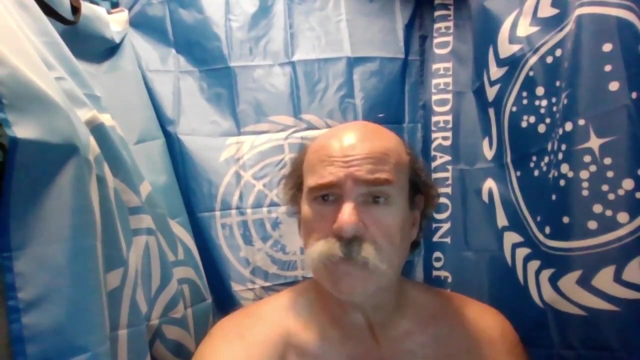 social sciences and artificial intelligence. Game theory is a tool for analyzing decisions, negotiations and strategic decision-making across a wide range of disciplines. By applying game theory models, we can make more informed decisions, design effective strategies and predict outcomes in complex real-world. 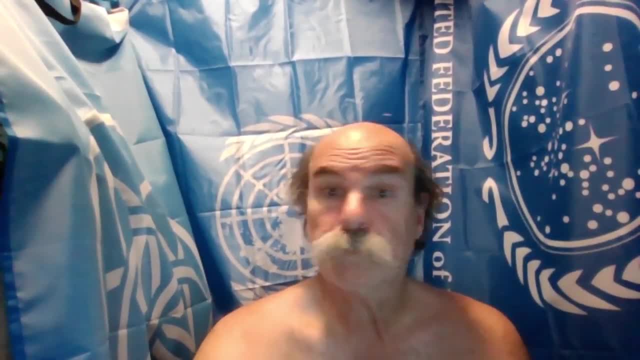 situations. However, it's crucial to acknowledge the limitations and criticisms of game theory. Simplified assumptions and the importance of applying game theory to complex scenarios remind us that game theory is a powerful tool but not a complete representation of reality. Its application. 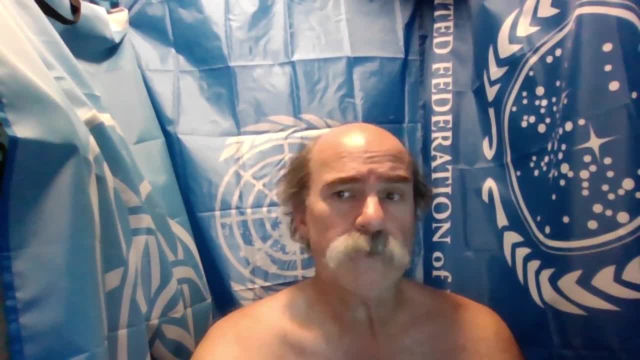 should be complemented by empirical evidence, contextual situations and the critical understanding of its assumptions. Despite its limitations, game theory has proven to be an incredibly effective tool. Its practical applications have provided valuable insights across fields shaping economic policies, business strategies.